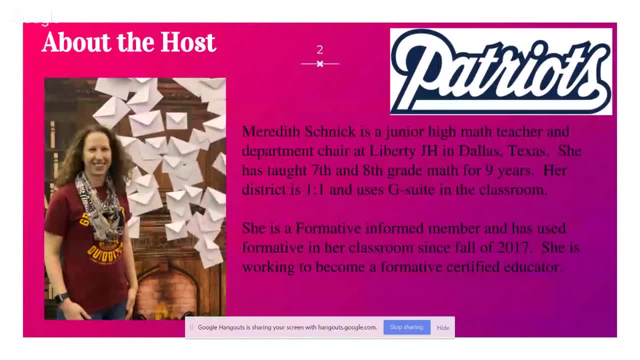 So our district is a one to one campus and we use a lot of our Google products, so it's G Suite, the classroom, all of the docs, Excel and the classroom as well. I'm a formative informed member. I'm looking to become formative certified. I'm almost there. 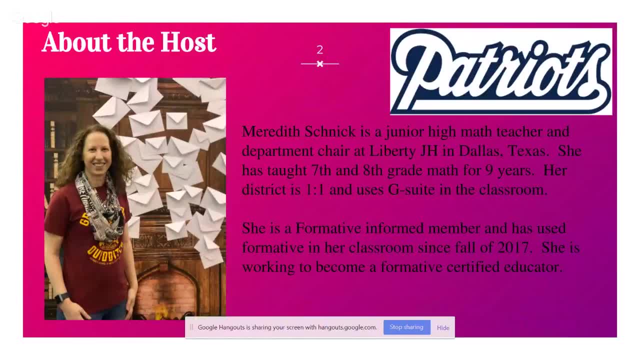 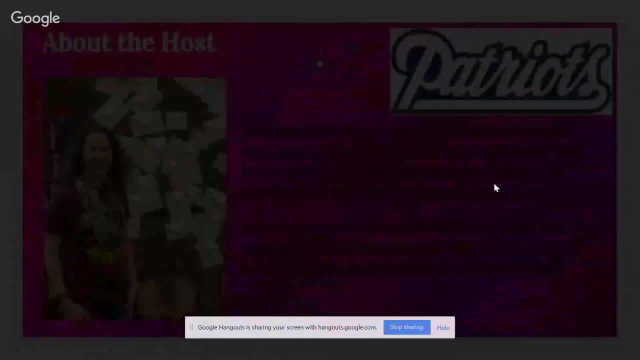 So right now I'm just going to start going over warm ups: how do you can use formative for warm ups and how you can use formative for the student activities and get them more engaged. So when I first started doing warm ups, I did the basic warm up. it was just I uploaded an image and it was a multiple choice question. 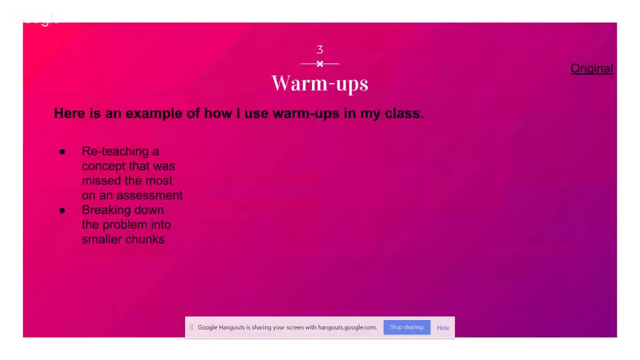 Eventually I started playing around with formative. They have a community center. That is so helpful. I discovered how to add links and videos to the what to the formative as well. So, doing that, I actually started doing reteach concepts for warm ups. 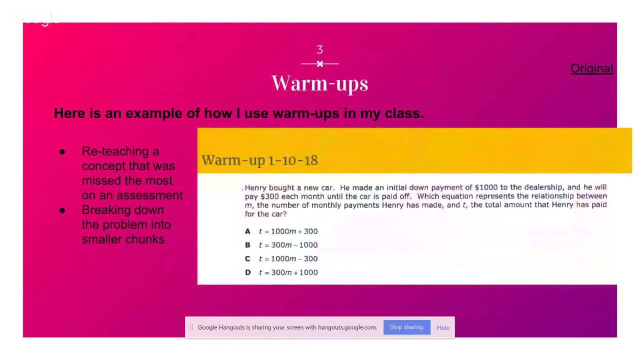 For example, this was from a unit test. this was one of the most missed questions And I noticed that they needed to break it down a little bit, so I started breaking the problem down into smaller chunks, So I love that formative allows me to break it down. 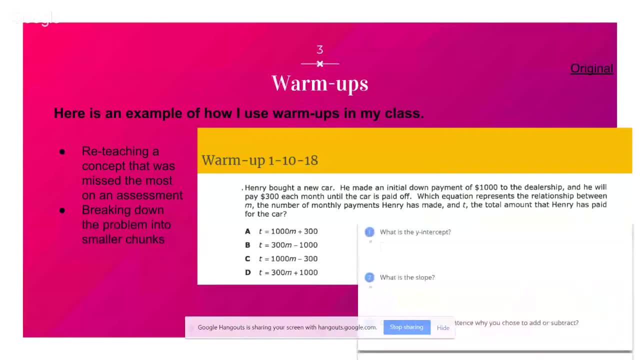 So I uploaded the little, the image, the question, And I was able to break it down for the kids and so they could see what they needed to do when they're solving a problem on a test or an assessment. So they were able to break down what's the y, intercepts, the slope, and explain. so a lot of it that I'm doing informative is having them explain a lot of their thinking. 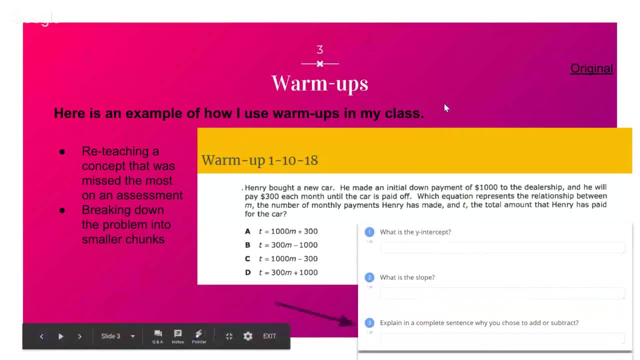 So, using this, I was able to see that most students- I was able to see that most students- missed this question because they subtracted, So they knew how with a y intercept and a slope was. but the main misconception or distractor for this one was they were subtracting. 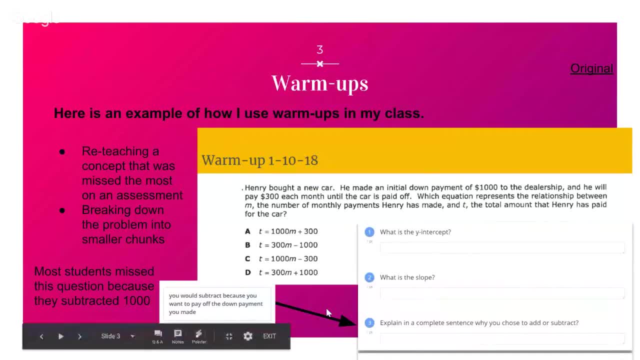 And so what I love about the explain is the students are able to explain in their own words why they chose that answer. I also love that it's anonymous, And so I'm going to show you an example of that involving the Pythagorean theorem. 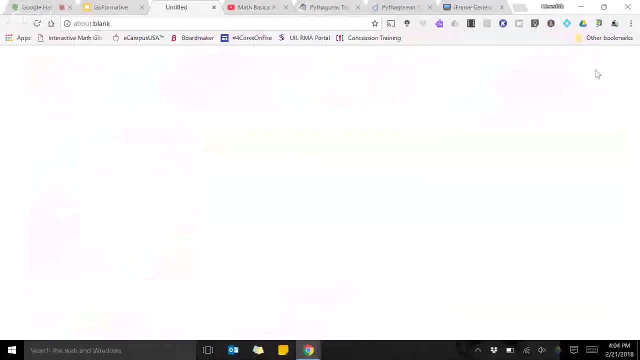 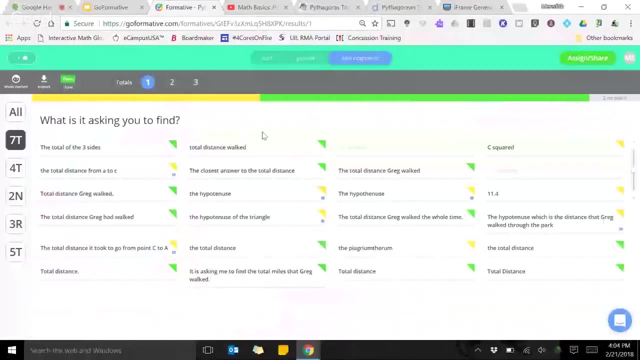 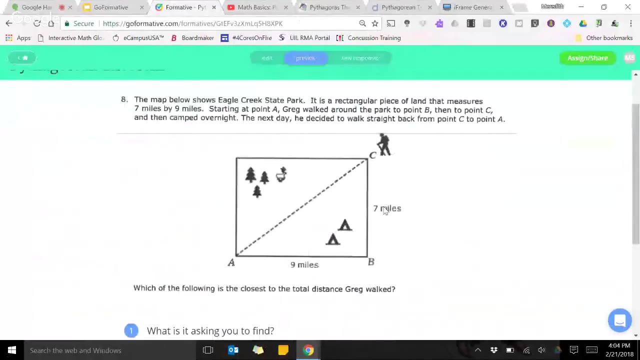 That my students did A while ago, so So on this one you can look. This is what a formative looks like, So I uploaded the image. so this was one of the most missed questions on an assessment they took And I broke it down because in the assessment it just asked which of the following was closest and it was multiple choice. 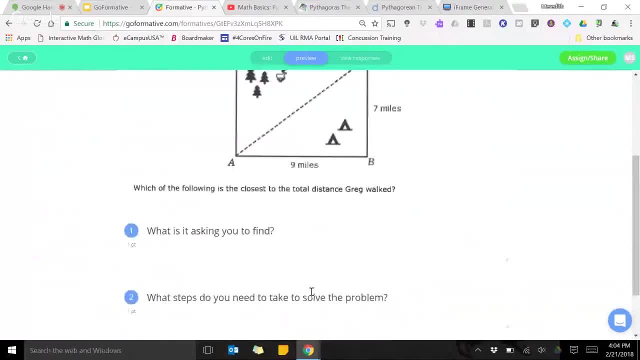 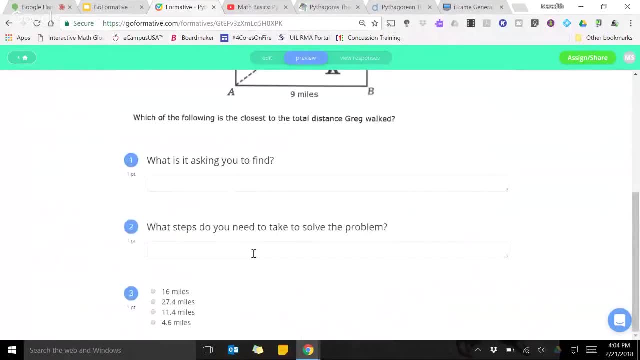 And so I broke it down into smaller chunks for the students to break it down. So what is it asking? to find? What steps do you need to take? And so, as the students are responding, I can actually go to where it says view responses. 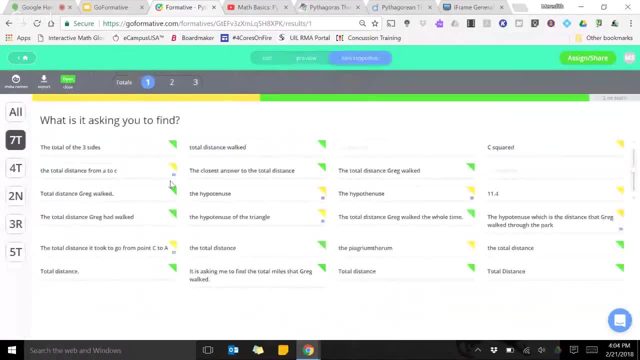 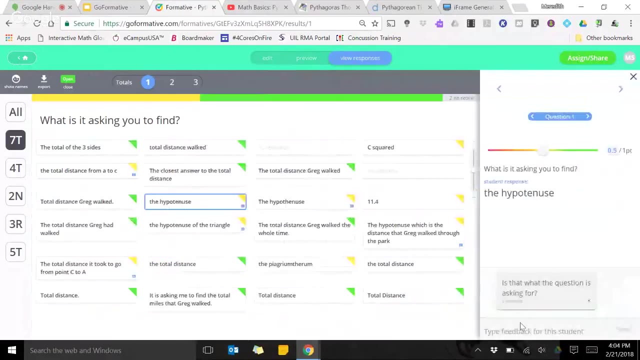 And it says: what is it asking to find? I can immediately see what the students write down. I can. It has little green or yellow. I can grade these right away. I can also go click on a name And I can actually type in feedback for the student automatically. 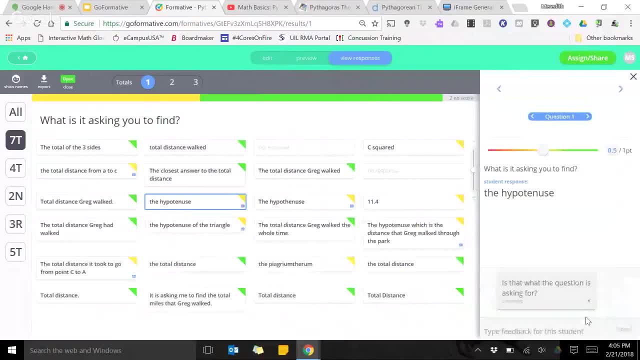 So the student: not only can I see the work, but I can give them feedback right away And they will know what's going on. So what I love about the warmups for informative is that students can respond. They know that I can see their names. 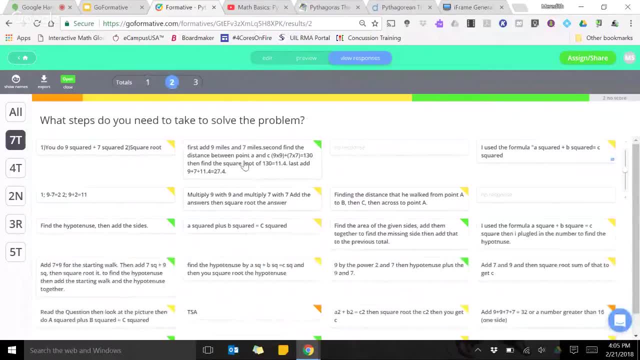 But when I show or project it to the class, I hide the names, So it's anonymous, And so they're able to see what other students are thinking or how they're working on a problem, which is one thing I love about formative. 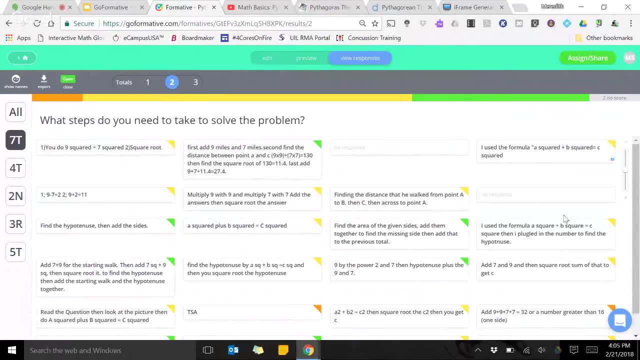 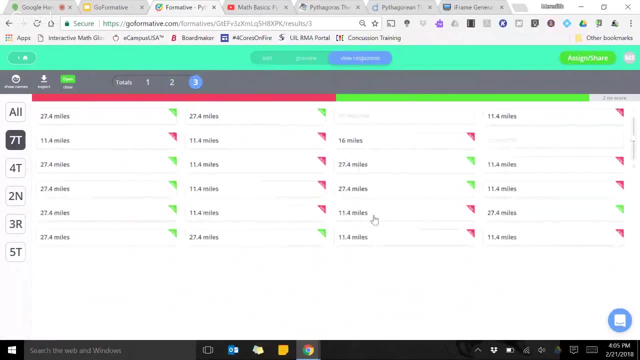 So I can just look and see how they're answering a question. So when I finally go to the answer, I can see which answer choice they're choosing- the most wrong. So I can see that they chose this 11.4 miles- And then I can go and see why is everyone choosing this as their answer, even though it's wrong. 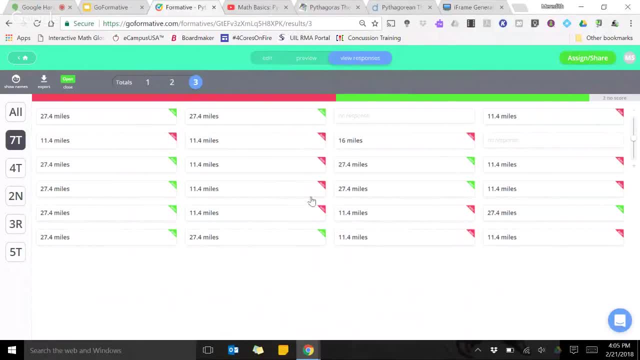 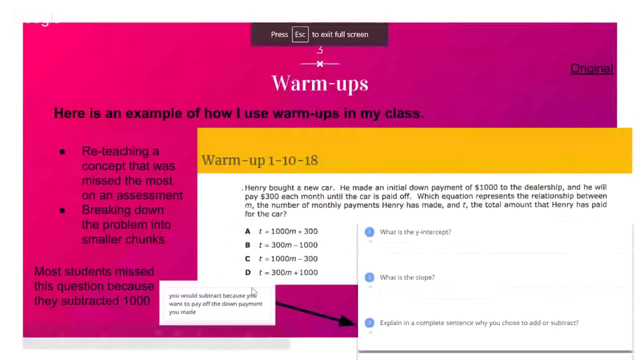 And we can kind of go over it right away and see it. So this is one thing I love about formative. I use this for warmups every single day, And so the kids love it. They know exactly what to do. They know how to log in and how to answer the questions. 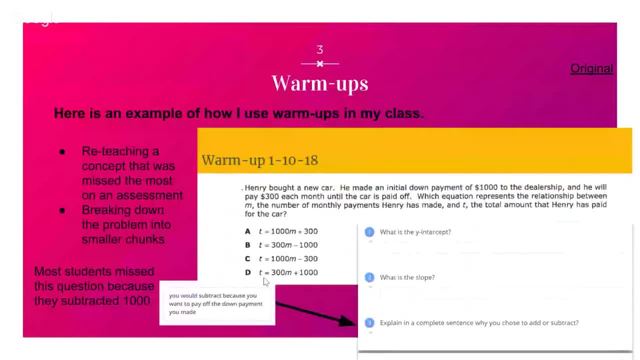 And so when I first started doing the explain, they sort of really small. I'm going to go into more detail later about how this has also helped with their explaining and going into more detail of how they were working out a problem, Because I first had to start with smaller chunks where they broke it down into small things, where they were just typing one or two sentences. 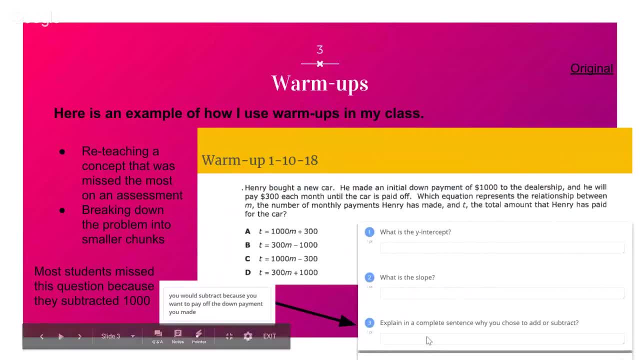 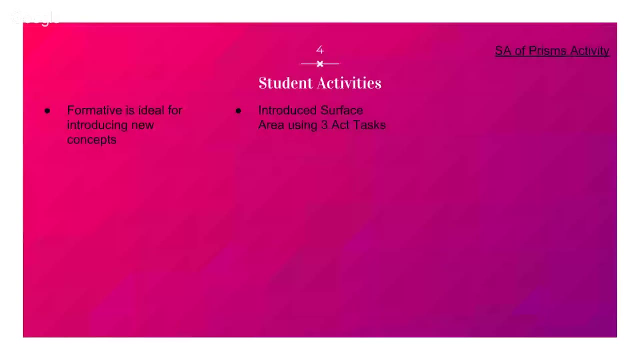 And eventually now they're writing About paragraphs explaining their work in writing. So that's what I use for warmups. In addition, I also do student activities with go formative. It works amazing for intro activities. I introduce surface area and volume using formative. 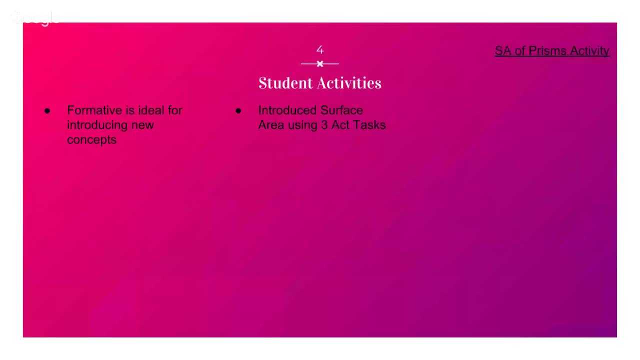 And I use something called. it's called three act tasks. You can find it online by Dan Myers. He creates these short little videos that the kids can watch And it Ask leading guiding questions for them. So I was able to Incorporate this, where I can insert a video with a watch. 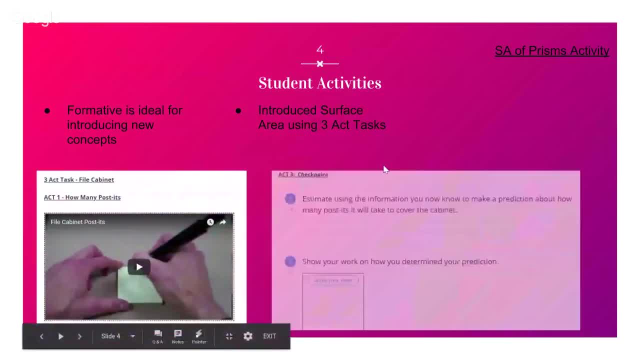 Then they can estimate. there's a show your work portion, which I'll show you later how to do the show your work. So the students can actually work out on their Chromebook and you automatically see it as they're writing. You can see on your computer what they're writing. 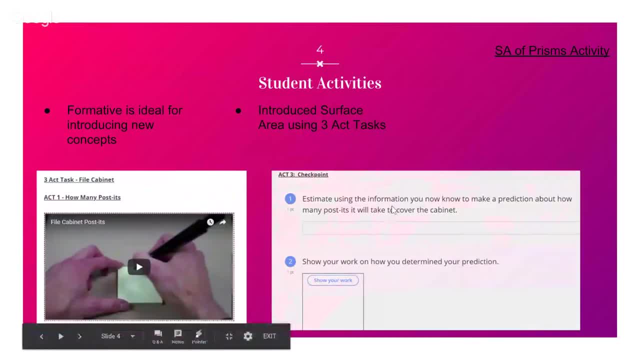 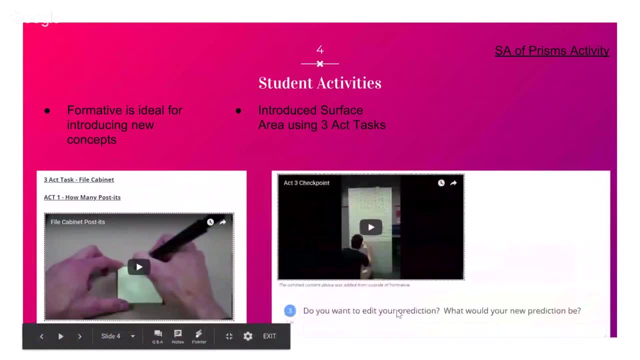 And then they had another checkpoint Where it added some more information. They get to make predictions about things. So this is an intro activity that I love to do And the kids get on. They're able to work and answer the questions. We kind of go over at the end. 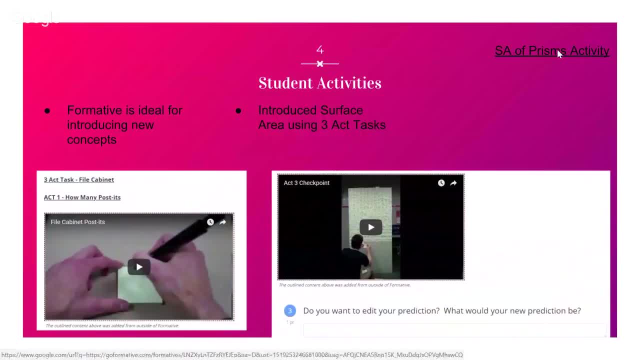 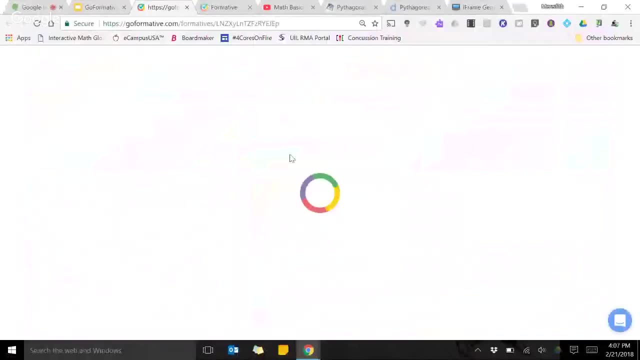 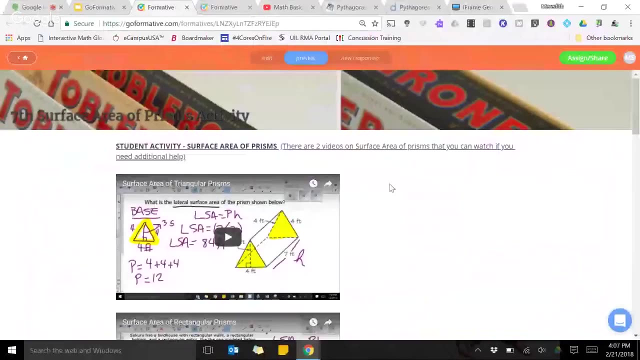 Another activity I did was the student activity. It's a prisms, So when you get on here, this is another formative I created. So this was: I did an intro to surface area And then we did a whole lesson And then by the third day I created this activity that they did on their own. 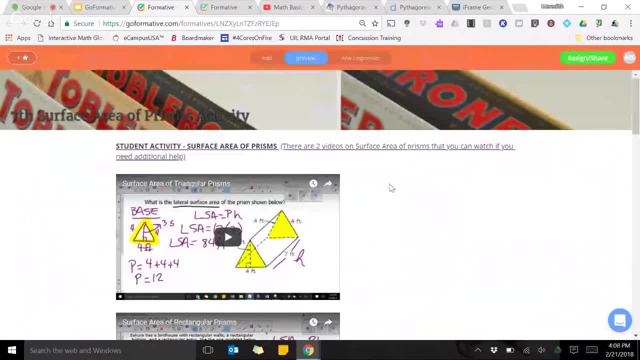 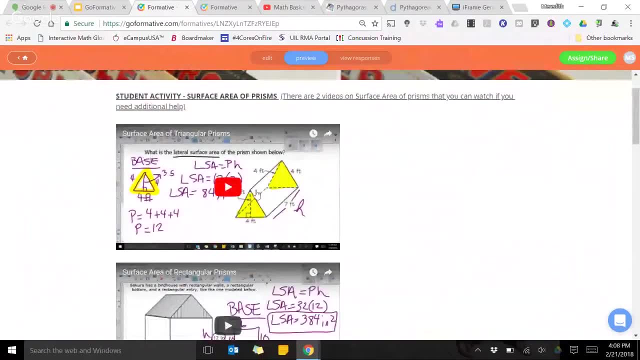 So they've already done the lesson. for students that needed additional support, I created these videos And it was able to embed the videos on the formative so they can watch it As if they need additional. So this had two examples: and prisms- triangular prisms, rectangular prisms. 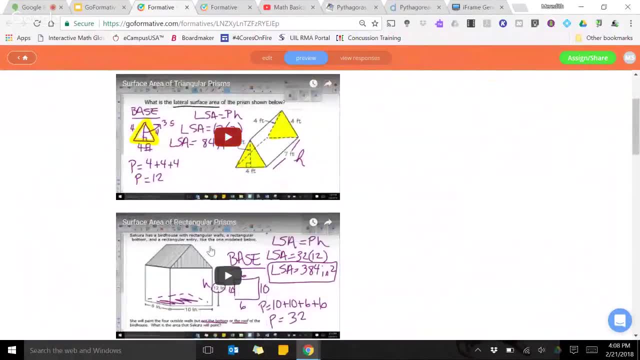 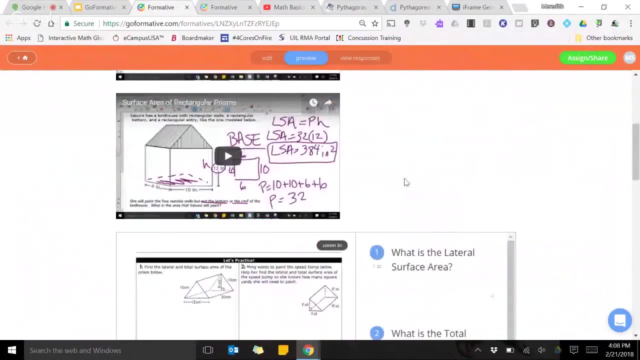 So if students needed additional support, If students needed additional helps, they could watch these two videos. If they didn't, they could just scroll down and answer these questions. So another thing I like about formative: it allows you to upload PDFs. 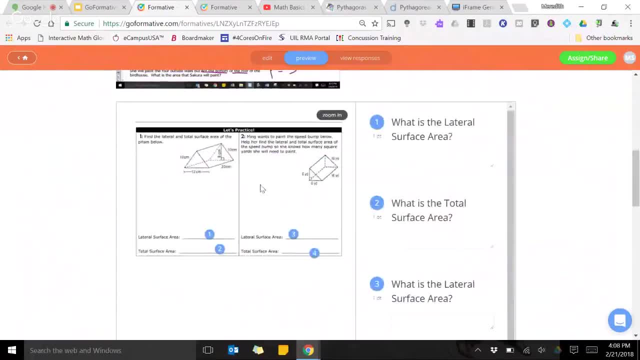 So I uploaded this worksheet And you can just click on as you're working. You can just click on whatever question they want You want them to answer. So if I wanted them to know that lateral surface area, they could just click here and total and put their final answers here. 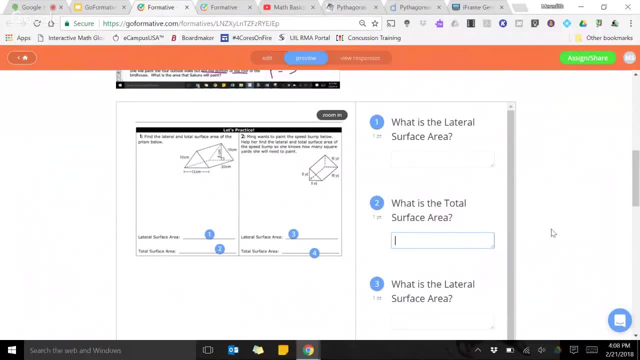 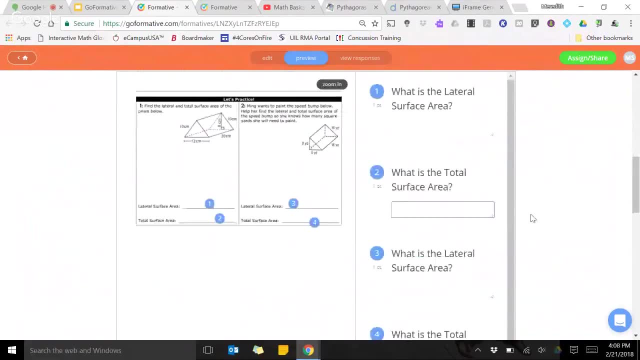 They did have the worksheet. I gave them a worksheet because I still think it's important For them to show their work, But then their final answer was on here And then. an additional thing that I did was they then took a screenshot of their image. 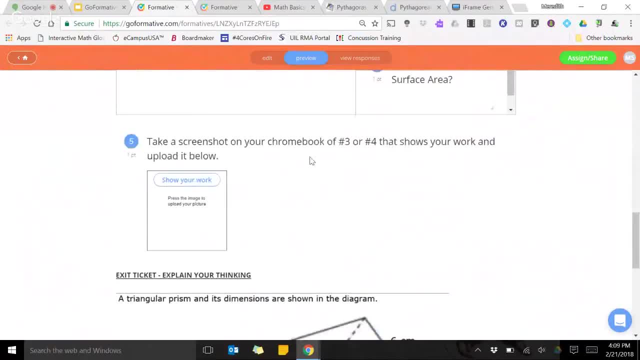 And so they got to choose between problem three or four, And then they got to upload on the show your work. So if you do the show your work, they could upload using this little icon right here And it's uploaded automatically. I can see it right away. 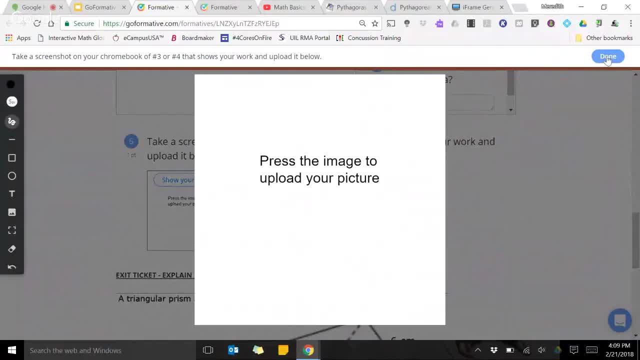 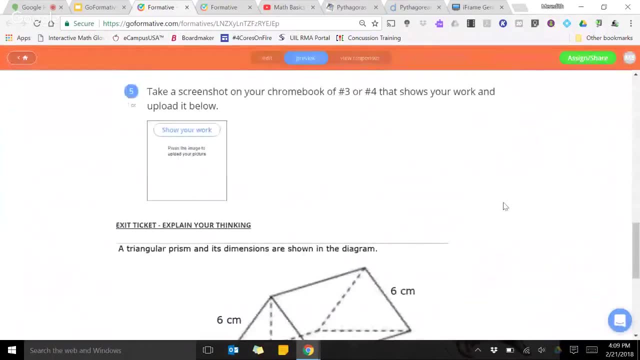 I can look and see what they've done. It's easier to grade, It's less paper as well. And then finally, I had a little exit ticket. So the whole entire lesson for the day was on the formative, So they did the whole video activity. 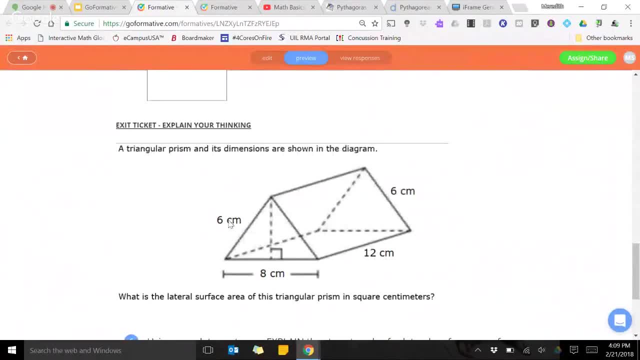 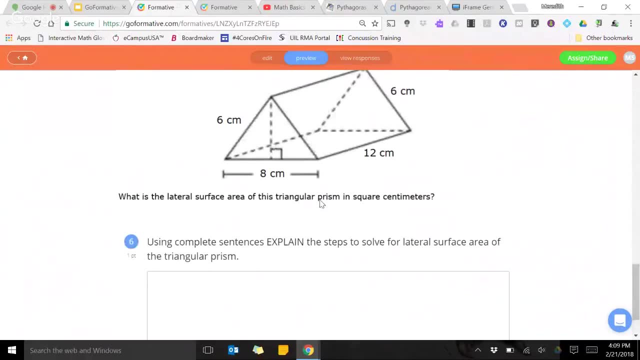 And then their exit ticket was also on here, where it's the explain their thinking So where they had to explain and write out the whole all steps for this. So this is another reason I use form at all time. It's just easy. I can do everything on here. 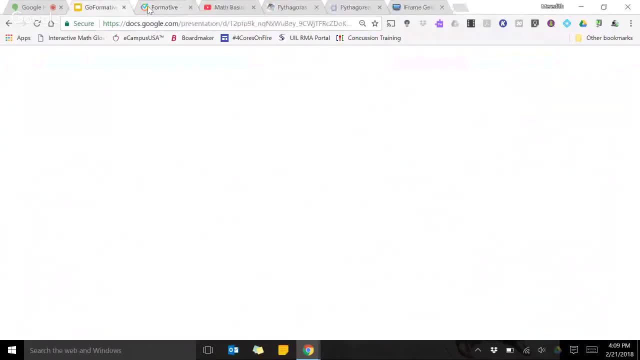 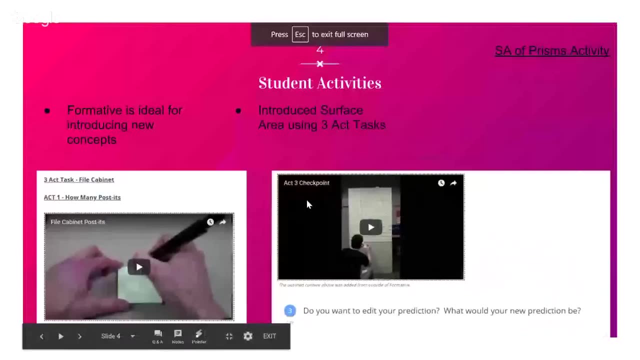 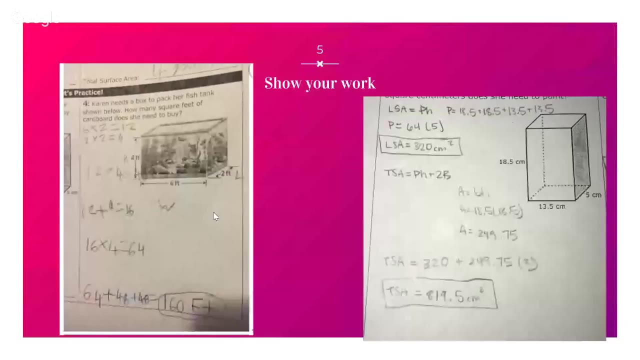 The kids find it easy to use as well. And then these are examples of kind of some of your show, your work. So a lot of times when I was talking about when they uploaded on the formative, this is what they're uploading, So they work out the problem. 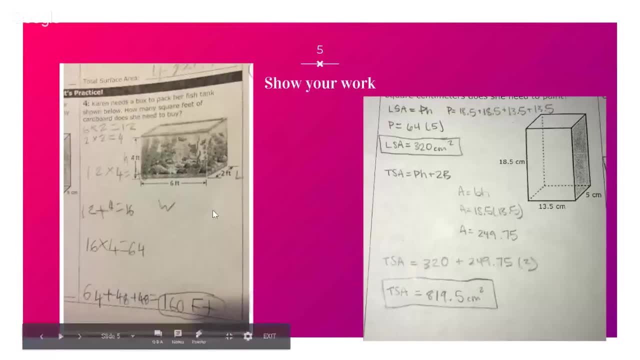 And then they're able to take a picture using their laptop or Chromebook and upload it. I automatically see it right away. I can tell if they're right or wrong. Again, it saves paper And the kids still get to keep their worksheet. 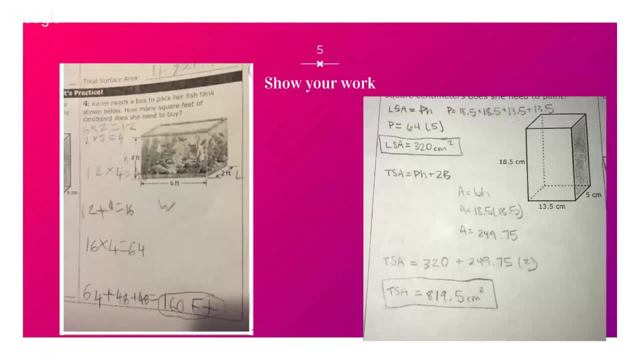 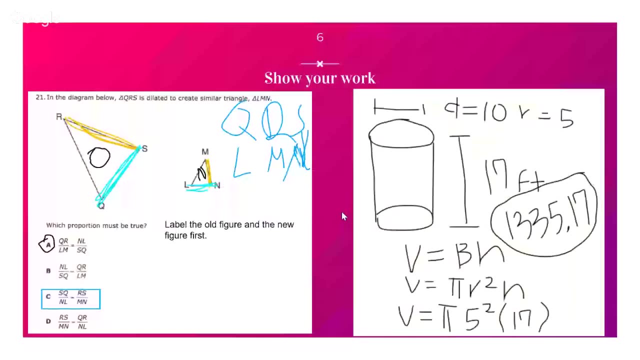 So if they need it to study, they can put it in their journal. This is another show your work that I did today. The one on the left is dealing with proportions, And so I had them label the old and new figure They drew on it. 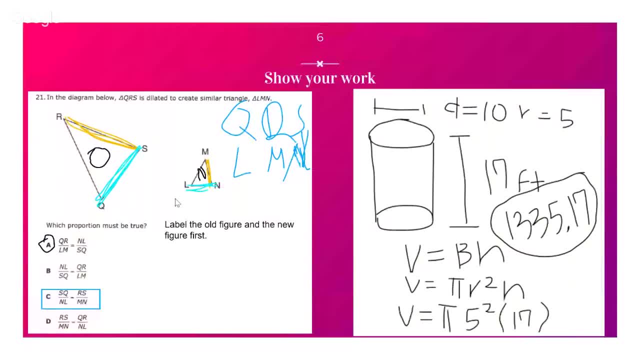 They circled their answer. I did have a separate one that actually answered the final answer And then the one on the right is on volume of cylinder. So the students were modeling out. They wrote out their formula And then they did And they substituted and solved for the formula. 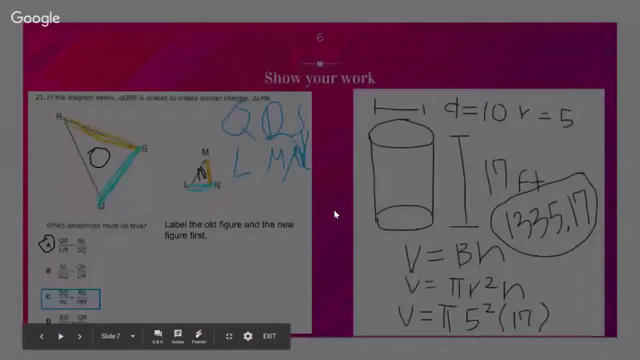 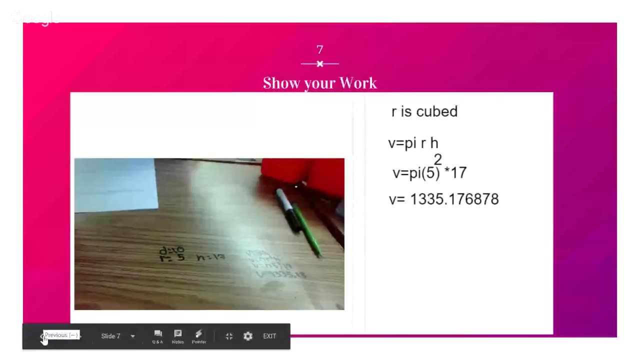 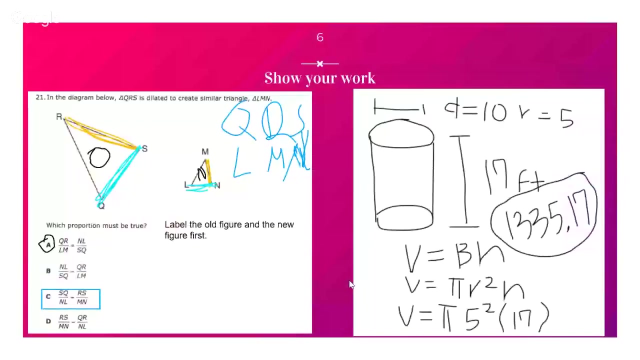 Another. Yeah, sorry, Oh, no, worries, I was just going to say that I'm loving the different ways that you're having students show their thinking here, You know, just as, just a quick review, Meredith is showing that you can have students, you know, upload images of their work in this, in this example right here. 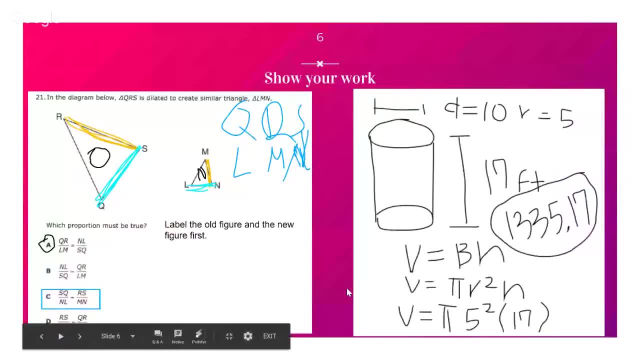 You see two different ways, which is really cool, She's- she's actually added an image of the problem. that image on the left, Right, And so students right on top of it annotate it to show their work. And then on the left, on the right, 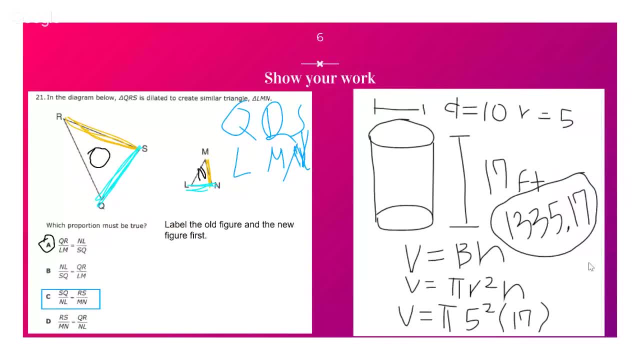 But I believe this is here is Meredith. It looks like you've just given your students, you know that- blank show your work Question and allowed them to draw their their response: Yes, And so this is where they're actually showing out their work, their steps, which I really emphasize: the formula and substitution. 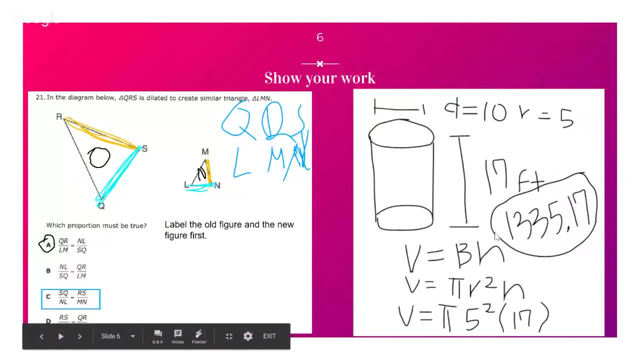 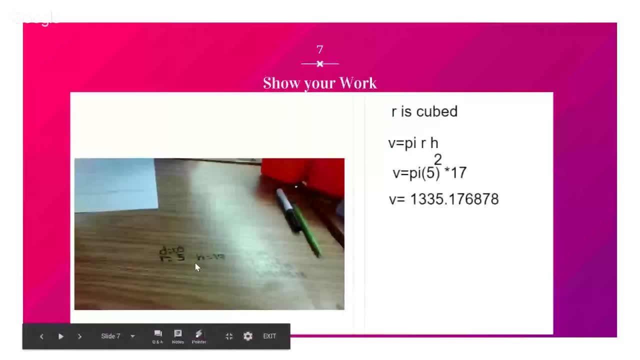 So they're doing all of that so I can see. And then on the next slide I had a student who actually wrote on the desk And he didn't want to draw it out. He didn't really like that using his finger or the stylus. 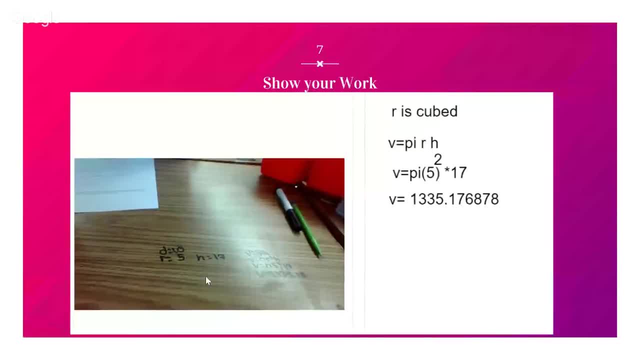 So he drew it on the desk with dry erase markers And then just took a picture of it and uploaded it. So there's different ways that my kids like to show their work and either draw it pictures. The student on the right actually typed everything in because there is a typing feature on the: show your work. 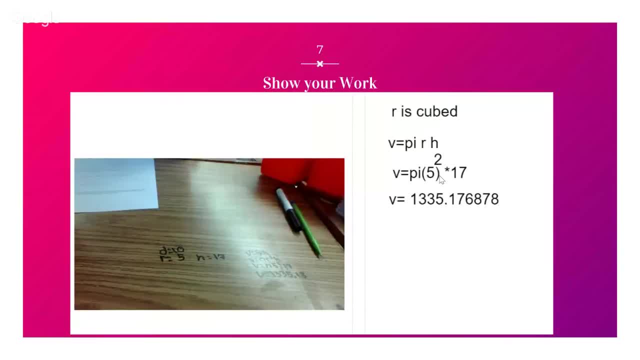 So there's multiple options for ways for kids to show their work. They don't always have to type, because I know it's sometimes they don't like to type or they don't always have to draw something, So I do like the different ways that it allows you to. 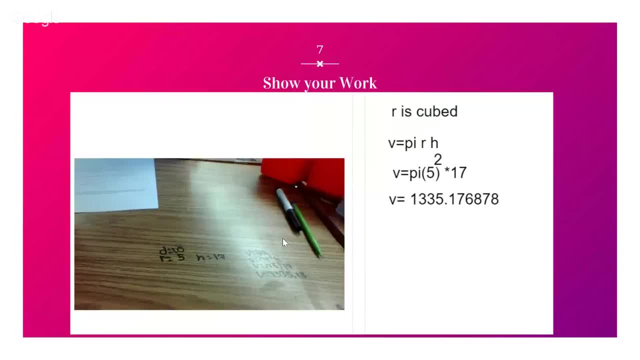 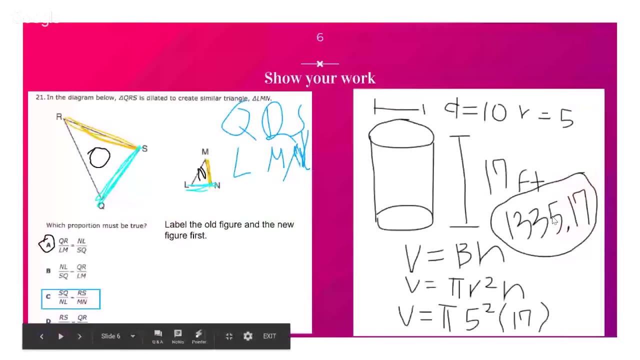 To have students show work. I also like that. it's immediate, So as the students are writing, So if they're, if I go back, if they're writing this, as they're writing it, I can see everything they're doing. So I can, I can look right away and see if they're doing a step right or wrong. 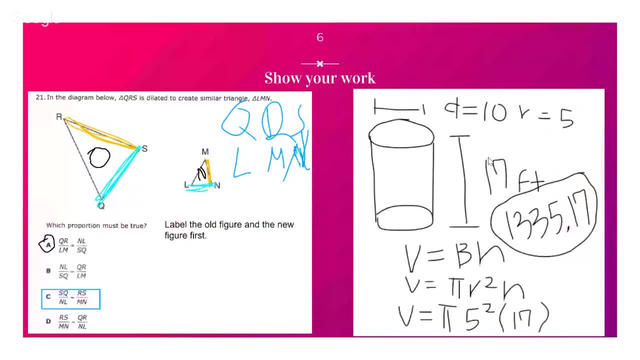 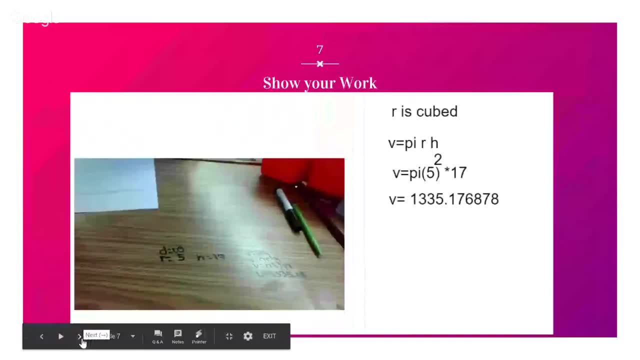 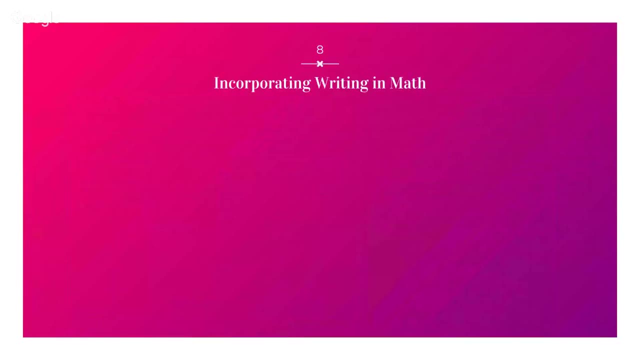 I can go and talk to them about it. So that's what I do love about formative as well. And then another With Our school is incorporating writing and math. So I've really tried to have students explain their thinking, Write out everything that they're thinking. 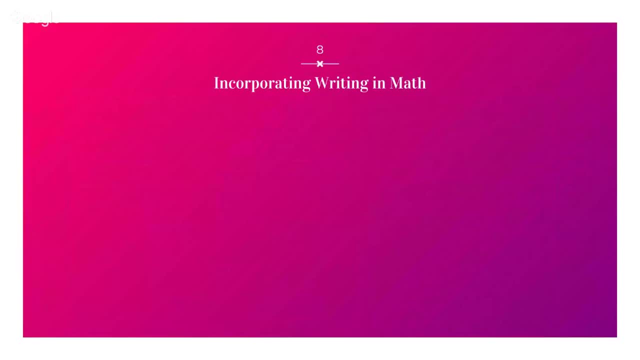 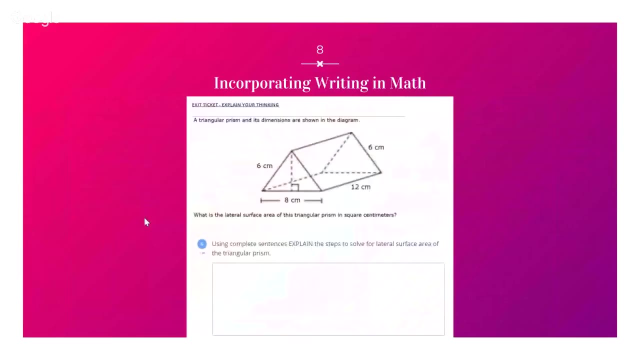 Why are they doing this? So I've started having students do. This is one of the exit tickets where they're finding the lateral surface area of a prism, So they solve for the prism first And then I had them explain The steps to solve. 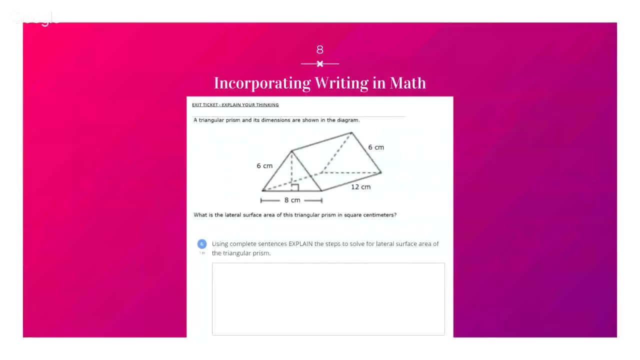 And I told them they needed to explain, as though somebody Who didn't know that much about math could follow their steps Step by step, And so Originally it took a little while, And so, when you can look at it, This is the example from the prisms that the students that are writing. 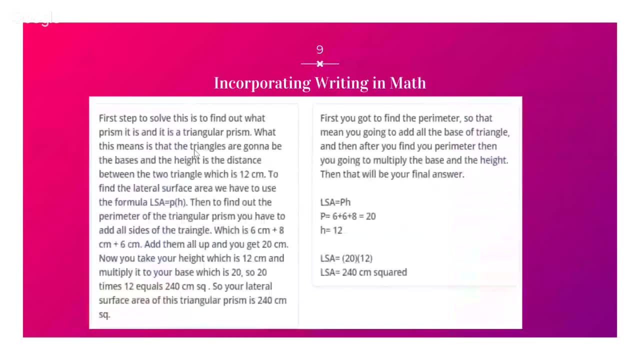 I had some students do whole paragraphs And as they're typing, you can see what they're typing. They are just explaining their thinking. The student wrote everything out. The student wrote everything out And then also showed their steps using the formula. 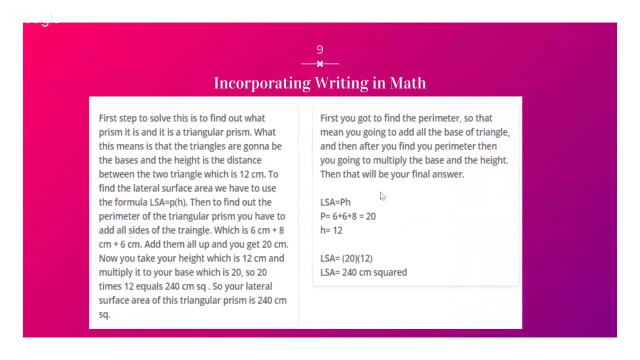 Which I like as well. So there's two different ways Of thinking And it's a process. It took them a while- Like I first broke it up into smaller chunks Before I went up to this longer- Explain their thinking Of writing. 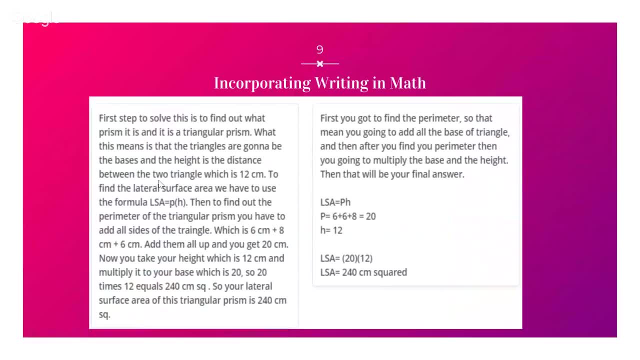 It's a. It's a huge thing, Especially in Texas We do. We have a lot of English language learners So they have to do Writing prompts that are sent off to the state And Also it's good for just higher. 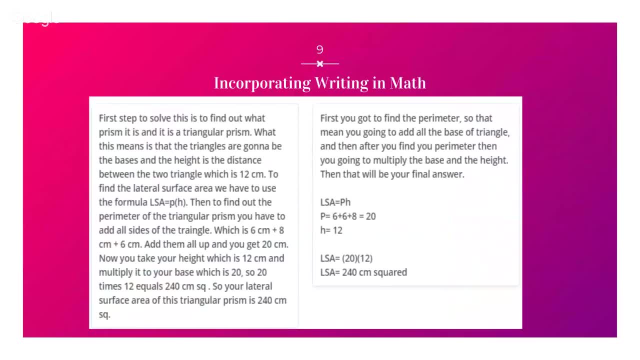 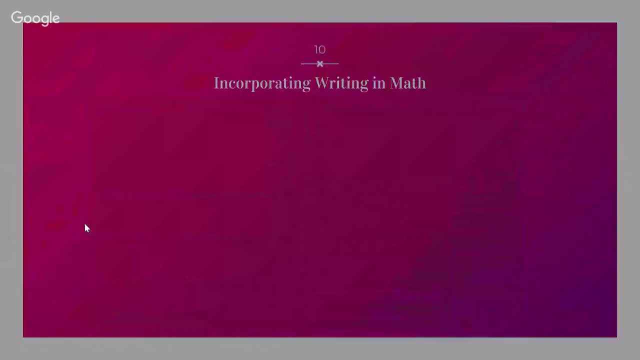 Think higher thinking Level learners. So Yeah, One thing I want to throw in there I forgot to mention was We're talking about this. If you guys want to ask any questions When you're watching over YouTube, Free to use the chat. 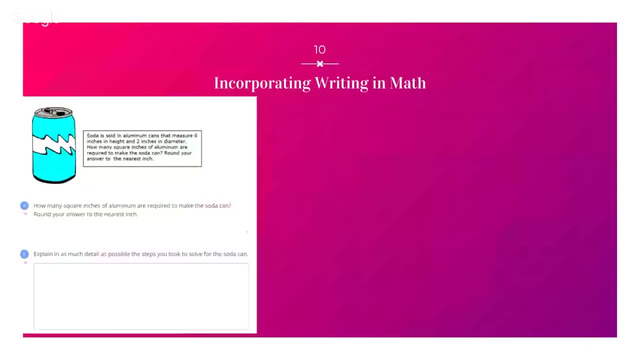 In the right of the screen and Leave your questions there. Then I'll check in a little bit Towards the end of the webinar So that we can address them For you. So any questions, Any comments that you have, We'd love to discuss them. 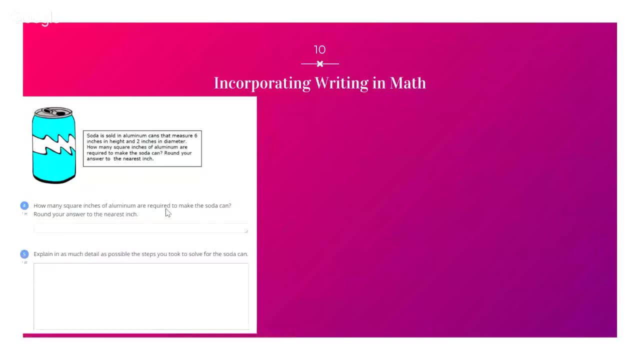 And then Also go over some of the examples Of how to incorporate the videos And the links and PDF At the end of this. If Y'all are curious about how I Uploaded the videos from YouTube And The images, 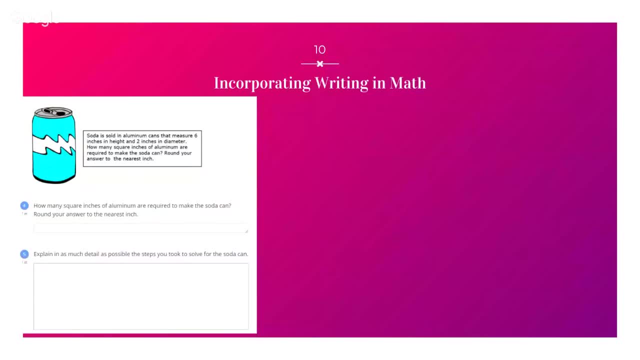 And I have another writing session. So If you guys have any questions, Please feel free To reach out to me. And If you guys have any questions, Please feel free To reach out to me. And If you guys have any questions. 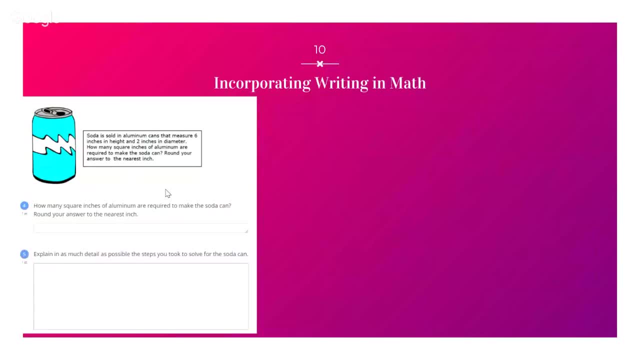 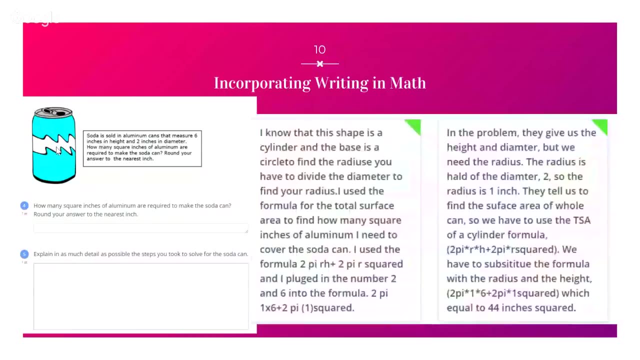 Please feel free To reach out to me. I have another writing sample That my students did. So they solved For the surface area of a Cylinder, And so It's not really about spelling At all. Like I can read, 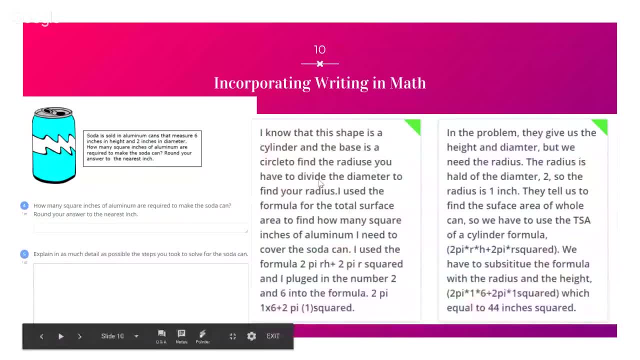 What they're trying to explain. So Getting them to start writing More is really important, And they started writing. That's what they expect For me now, And so When they come in And I do the formative, They're not surprised. 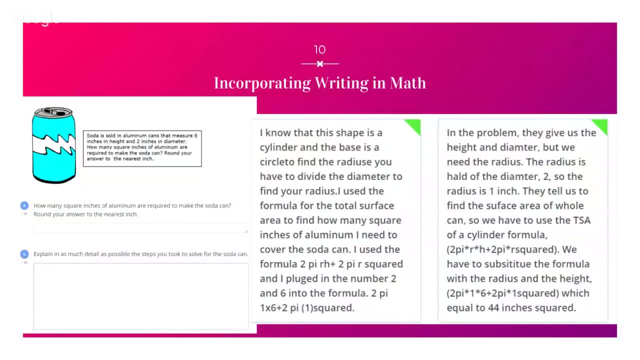 I also think that the typing Helps a lot With a lot of students, Because i'm finding students don't like to write because they either can't write that well or they don't really know it kind of hurts, so they don't really like the writing as much. 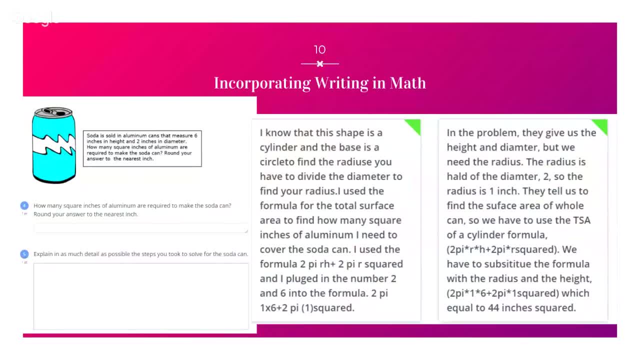 using pen and paper or paper and pencil. so i found that having them actually type is a lot easier for them and they're more willing to go into more detail if they're typing. so that's another thing i like about formative: it gives that typing option with your explain, explaining their thinking. 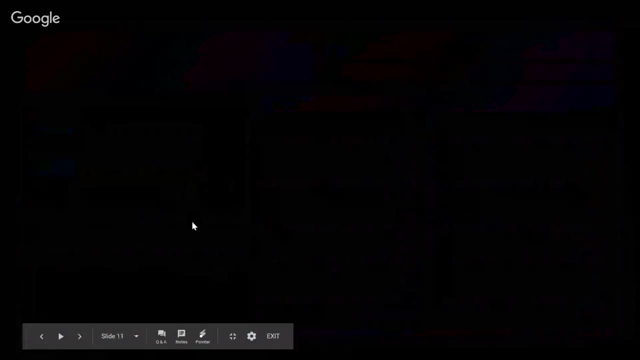 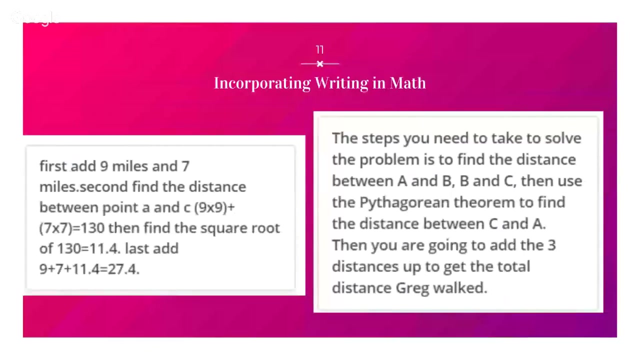 so here's another example of incorporating writing in math. this one had to do with the pythagorean theorem, so they had to explain the steps to solve for this problem and again, kind of, some students are still trying to work towards the writing more, but they're. 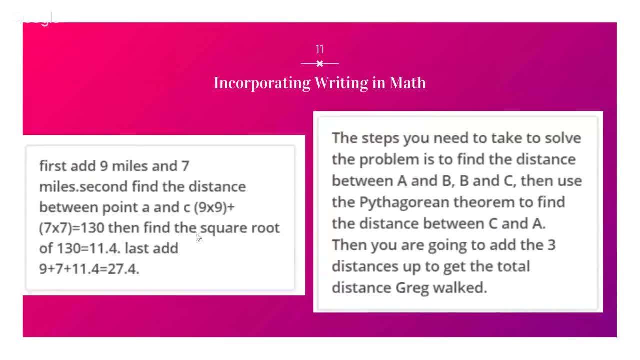 still showing their thinking that i can understand the process for how they're getting their answer, which helps me to know if they're getting the point or if they need to be retaught or there's a little thing that they need to be, uh, fixed, a little correction. so now i like to go over just how i make the formatives. 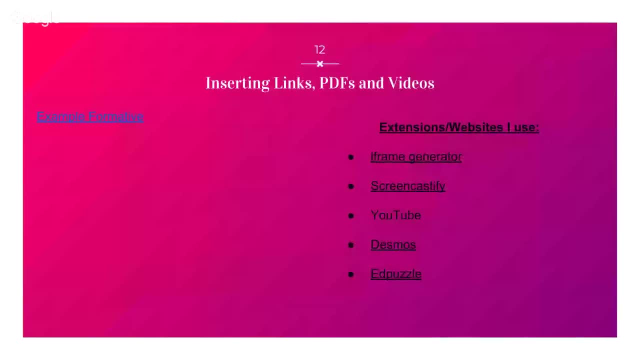 because they're really easy. they don't take that long. when i first started making formatives, all i did was do an image and a multiple choice, so that's what i started with, and after i got that down, i started introducing videos, the open-ended questions and the show your work. so it does get. 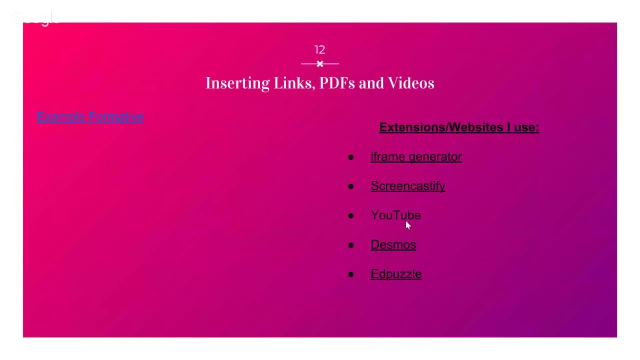 easier. these are some extensions on the right that i use that i'm going to go over. i use this iframe generator generator that i'll show you in a minute to embed a website within formative screencastify. i'll go over that in a minute. is just a way that you can record your screen, if you. 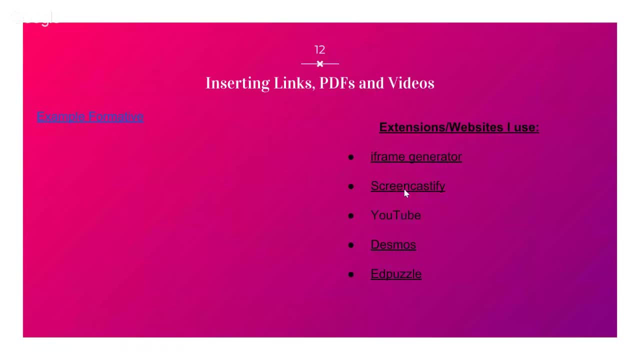 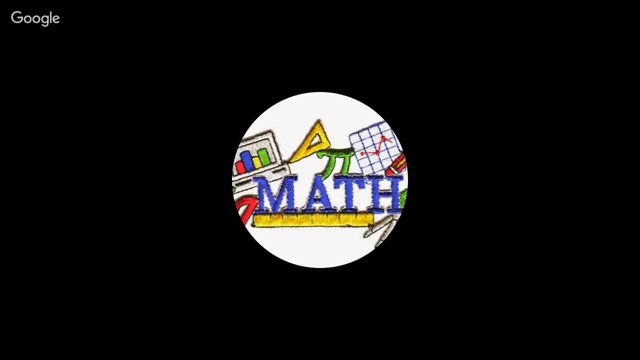 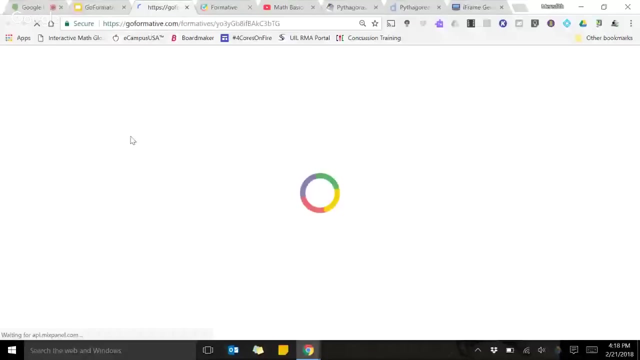 make videos. so this is how i make some of my small four minute videos for the students. and then these are two programs i use. i use desmos a lot with. this is a graphing i. i just go to the formative. you can give it a title. so i gave it the. 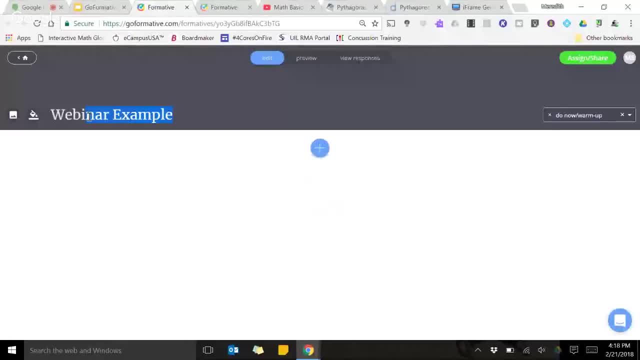 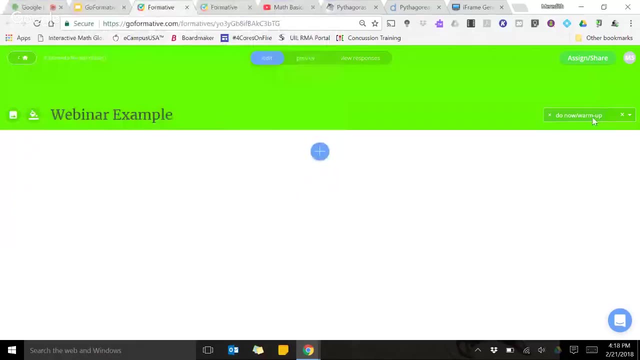 webinar example. you can. you can change it if you wanted to. you can even change the background color and eventually, you can even add videos- uh, not videos images- if you wanted to. you just have to find the correct scaling for it. so, and then you can label it, which i love, as well as either an exit ticket- i'm going to do this as a 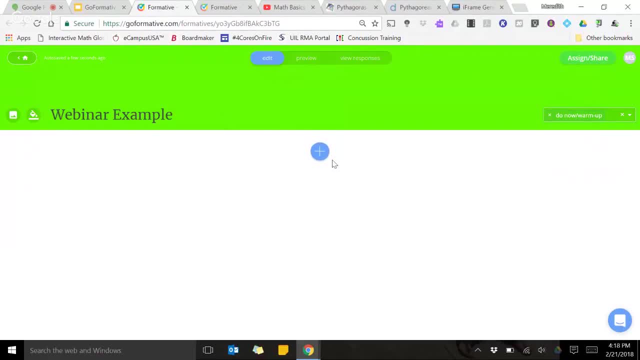 warm-up. so one of the first things i would do if they i was doing a lesson is introduce it with a little youtube video if they needed extra help. so you just hit the little plus button, which is easy. it gives you a list of options. so i want to add a video, so i'm going to add a video. 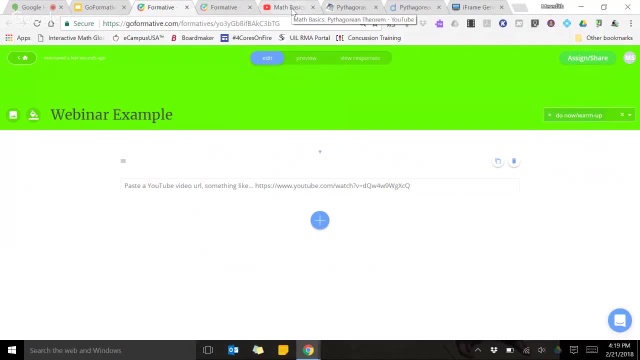 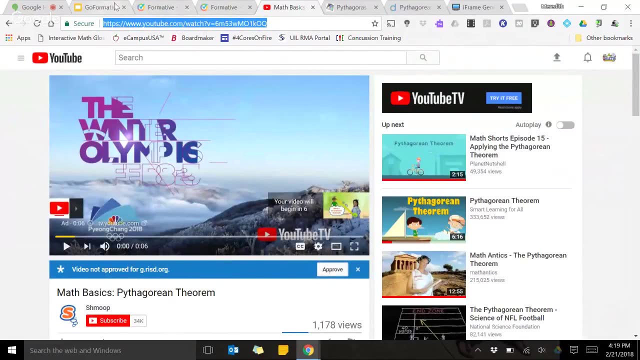 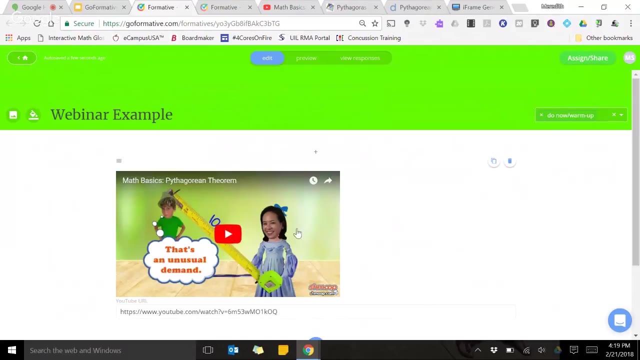 from youtube, so i would just go up here where to my youtube. i'm going to do one on the pythagorean theorem. so all i'm going to do is copy the link, go back to my formative and then paste it in and you just have the update and right away it's going to update and put it in. 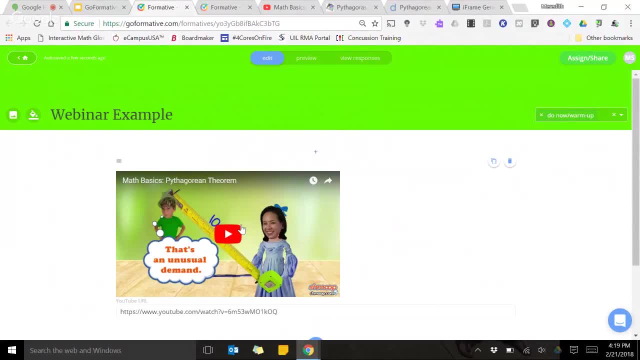 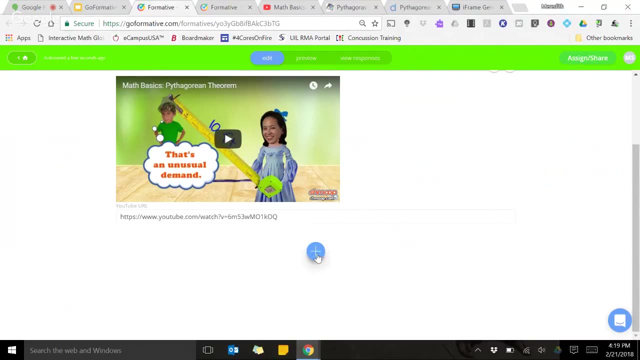 your video in the formative- just so easy and you just hit play. the kids can hit play. it plays right there on the same screen. it doesn't open a new tab, so that's what i love about. you can insert youtube videos. another thing i like is when you can also do links. so, for example, if i wanted them. 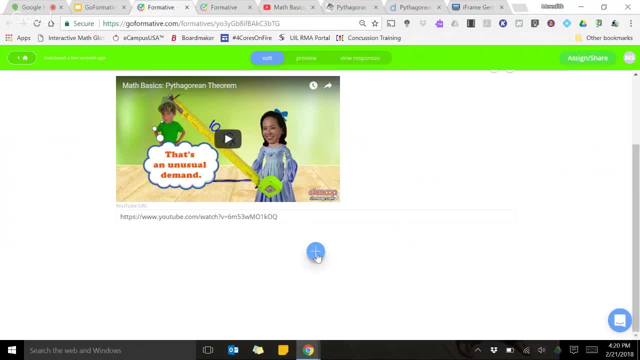 to have additional information or a definition about something, you can add links. so if i wanted to do a text box right here and i can just say you will be doing an activity on the pythagorean theorem, so i want to do a link so i can actually link, hyperlink these words, so i can go. 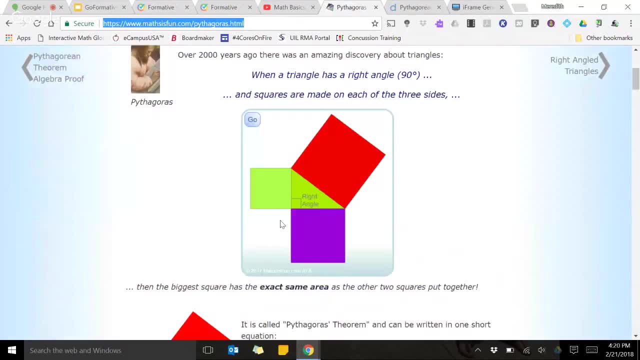 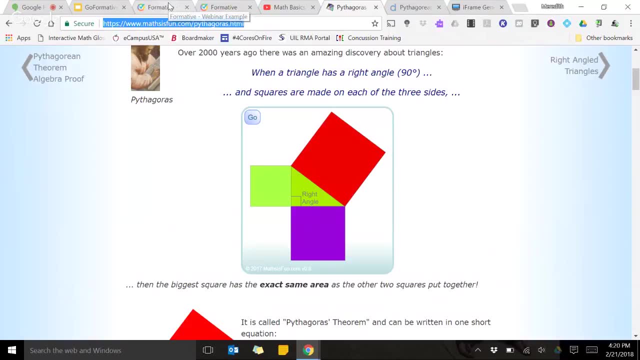 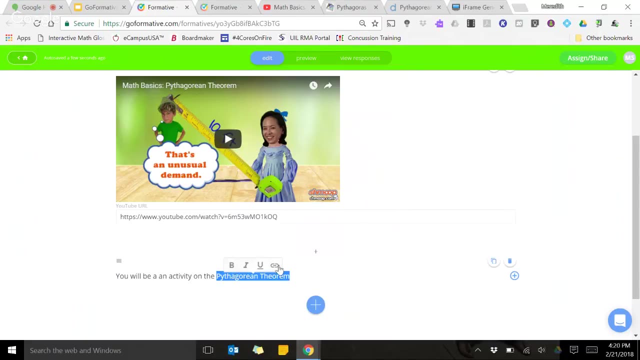 to this website, which gives a definition of a pythagorean theorem. i just copy the website. i can go back to my formative. if you highlight whatever you want to be hyperlinked as soon as you highlight, this comes up. so even if you wanted to, you could also bold it or underline it, so it gives you that option too. but you're going to do the. 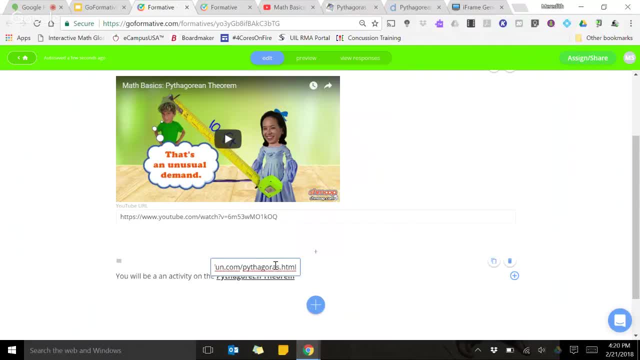 little chain and you just paste in your hyperlink and you press enter and now it's hyperlinked. so when you click on it you can see that it's hyperlinked. and you can see that it's hyperlinked. if you click on it it will open up a new tab and they can go and read about the pythagorean. 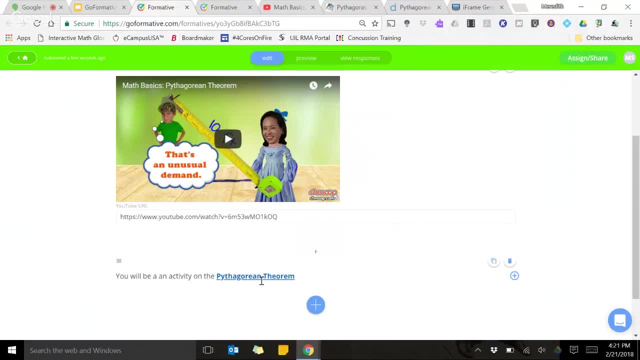 theorem. so if they were still struggling with the video and they needed additional information, they can go back to the link and read some more information about it. so that's what i love about formative: it has all these options for kids to get different levels of instruction. 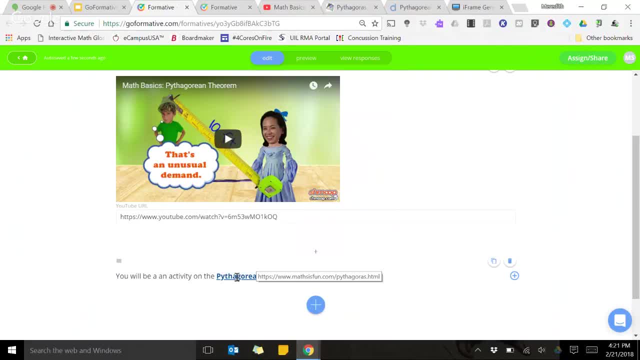 if they needed it. awesome, meredith, i just had a quick thought as well. um, so i was just uh gonna mention um, so you can actually give you know instant written feedback with formative as well. i know meredith pointed that out, um. one thing i love now is you. 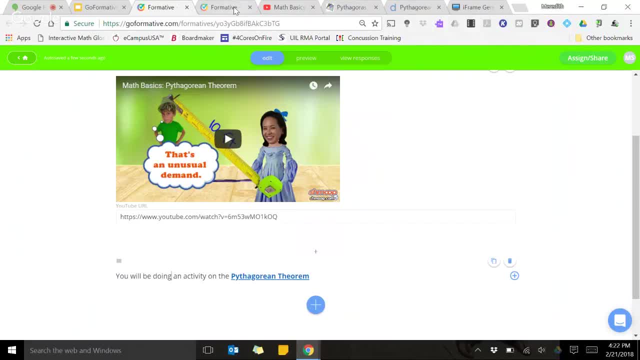 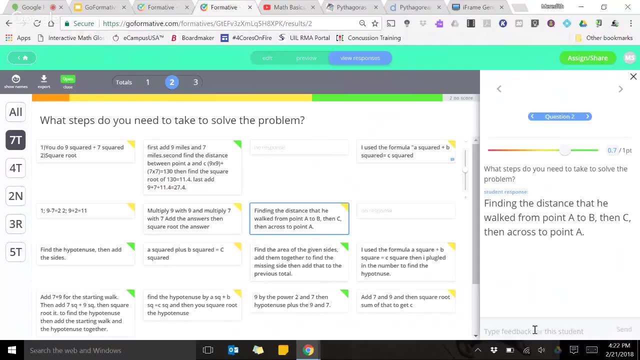 can hyperlink the feedback that you're giving. so, yeah, you know, if you want to give students- not only just you know- a written message, um, you can. you can also send them to a personalized resource that will help them. so like, for example, if you're noticing that you know this student is. 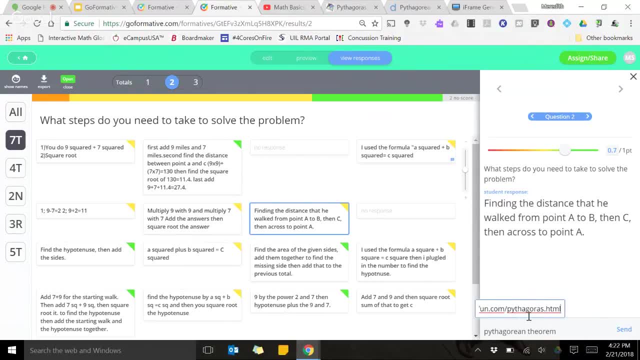 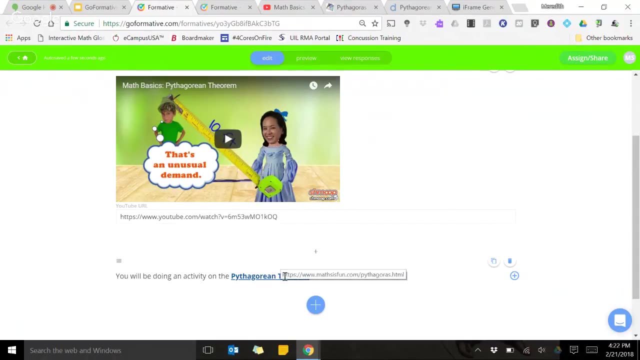 struggling with the problem. in a certain way you can, as meredith is showing you know, send them to that specific place. um, personalized help, yeah, so it's really nice. so that's why i love the links, and the kids know that anything that's in blue is a link. now, so they 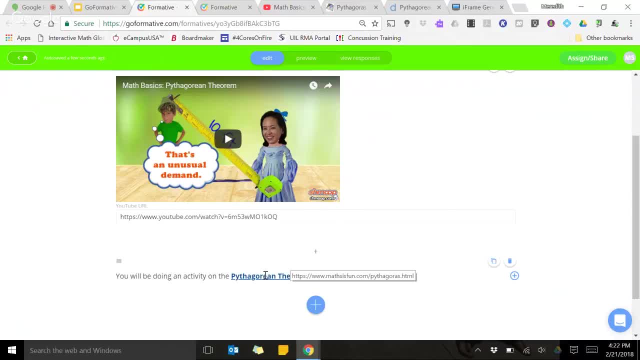 don't even ask questions. if they see a blue, they know it's a link because they they're used to it now. in addition, sometimes i don't like having kids open a bunch of tabs, so if they're clicking on a link it opens a bunch of tabs. they might delete the wrong link or they're formative. 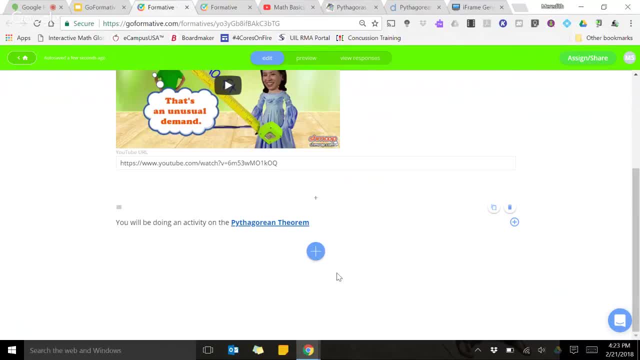 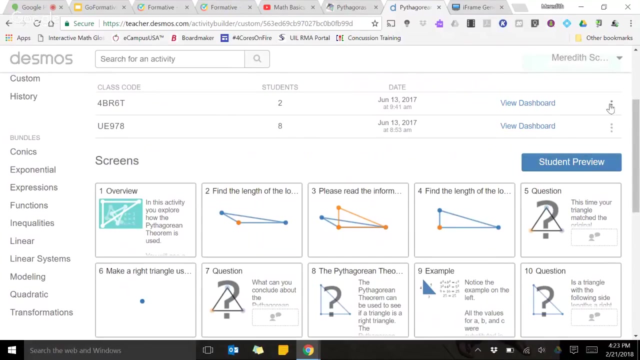 so what i like to do is embed a website within formative. so you just add another content. so i go to this embed thing. it says embed, so i go to it, and so i want to embed desmos within the website so i can go to desmos. this is the link. 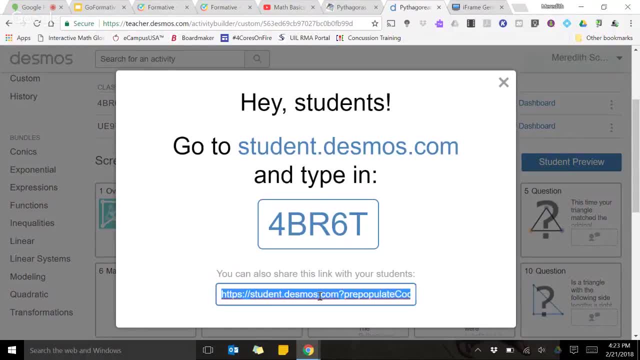 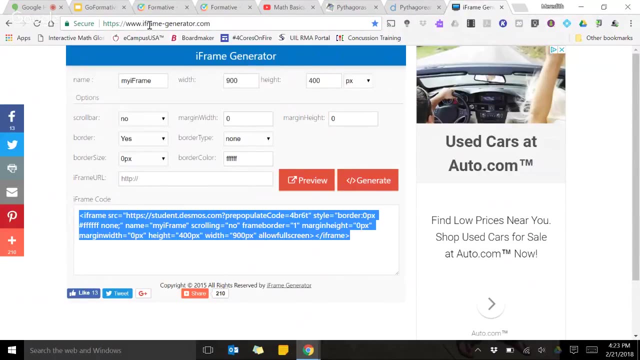 i want to link the student link right here, so i'm going to copy it. i go back to my formative. sorry, so another. so i copy the website. i use this uh website called iframe generator, so if you just look it up you can go to it's called iframe generator and you just paste the website, right. 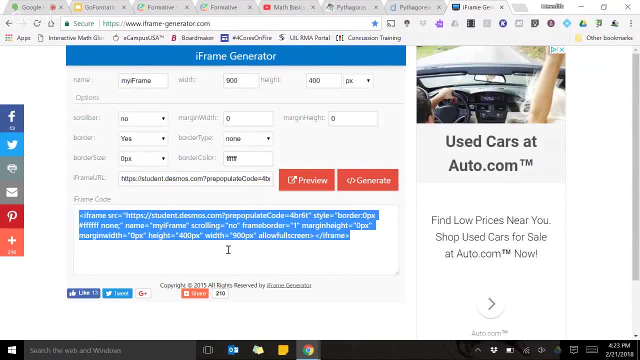 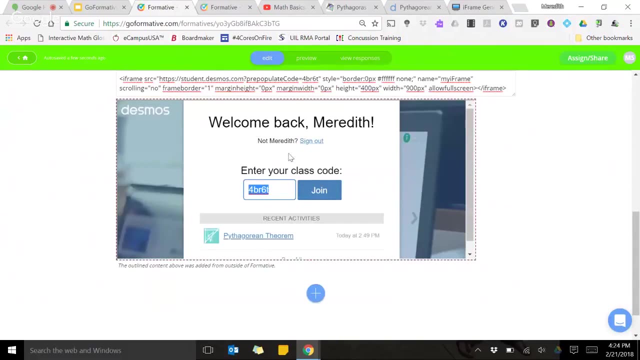 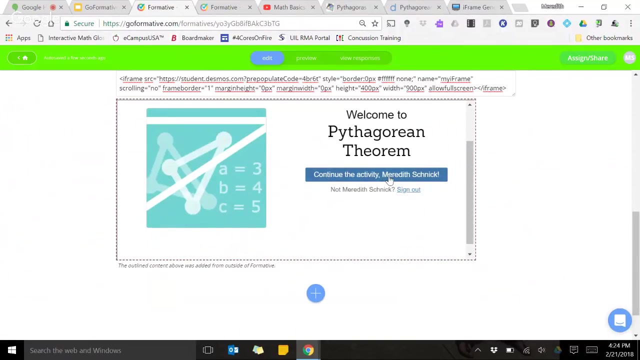 in here and you hit generate and it will create an embed code for you that you can just copy and then paste it into your formative. as soon as you do that, it will come up. so everything the website is within formative. so if they want to do the formative, they just hit and they can continue with activity. 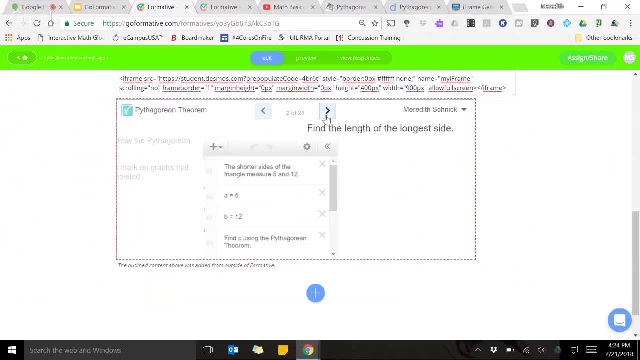 and so the whole activity, the whole website is on formative, so they don't have to open a new tab, they don't have to go and figure out which tab do they need to do, because it's right there again. if you wanted to, this is kind of small, you can also change. 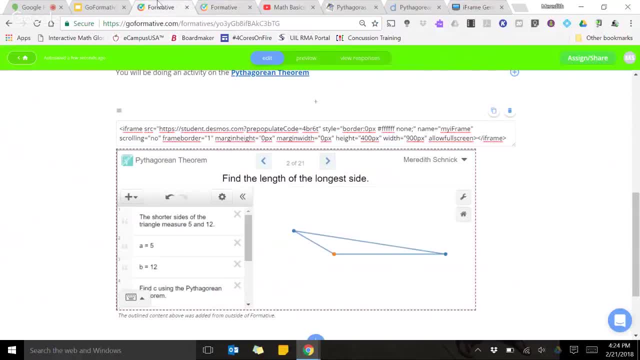 the width and the height. if you go to the side section, you can just click on the tab and say, okay, height. if you go back you can change it as well. so this is one thing i love about formative: that it has this option to bring in websites or other programs. so if you wanted to do an ed puzzle, 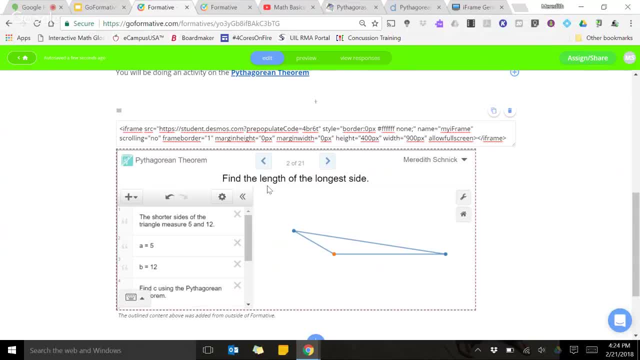 or if you want to do something on khan academy, they don't have to open a new tab. they can do it right within formative meredith. um, just a related question, dean. uh, one of our certified educators actually was watching out there and was wondering: um have you? 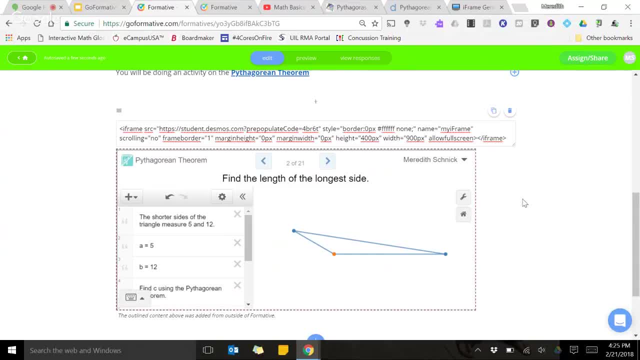 ever tried embedding geogebra into your formatives? i have not actually, so i i'm thinking it it may work. i'm not sure. i i actually haven't used geogebra a lot. um, i use desmos a lot, but i wonder it. i'm assuming it would work if it's the same process as. 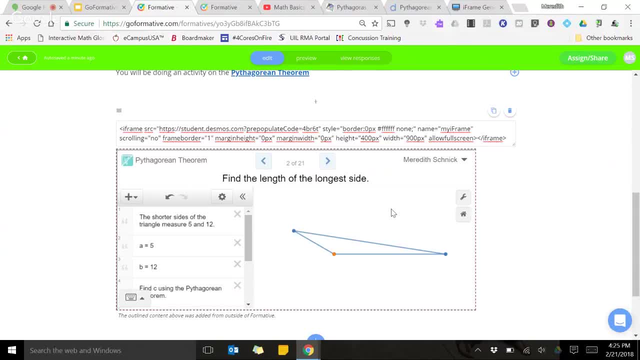 the desmos. yeah, it's, it's good, it does work. i think, um, there might even be some examples in the community center of teachers using geogebra. but just uh, that was one of his recommendations, and then uh, or just one of his questions, and then another one that he had i thought we could bring. 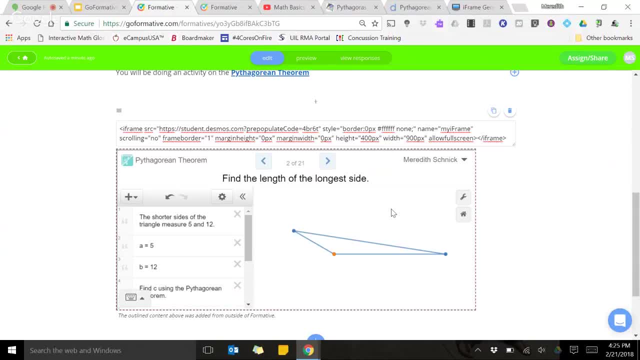 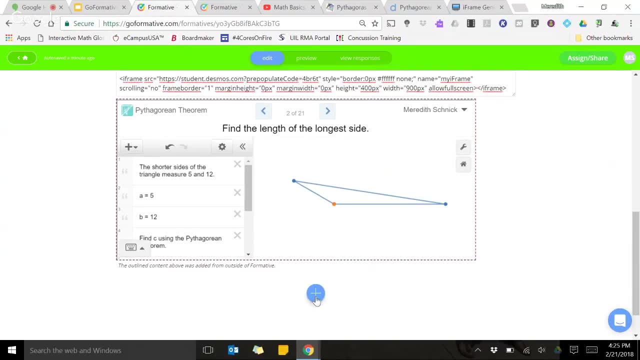 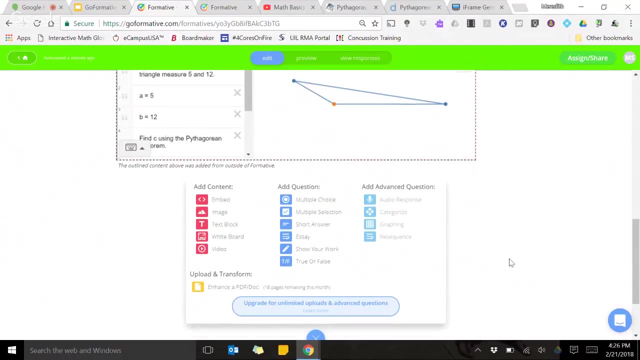 up at this point was: he was wondering if you've ever tried the audio question type before. oh no, i haven't. uh, i haven't, so i'd be really intrigued. i'm actually really interested in using it, the audio. where is it? oh, the audio response? no, i haven't used that. yeah, he was just. 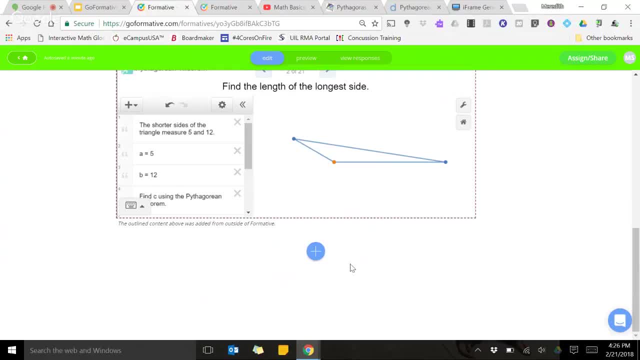 mentioning that you know like, in addition to having your students write out their responses, just the audio could be another way for them to explain. yeah, yeah, that would be nice, because i know some students would like something different besides writing out everything all the time. so that would be an another option, because i know that if they're explaining it, they 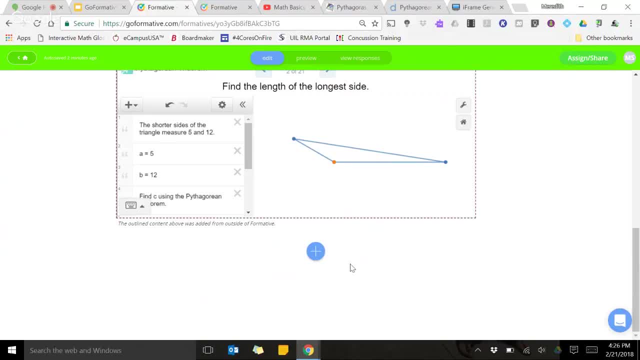 feel more confident uh explaining it verbally than writing it down. yeah, definitely, i think it's a great uh modification. and just one more idea to throw in there is: have you ever heard of uh? have you ever heard of uh speak pipe before? oh, no, no, i haven't what. i know that uh, we've used. 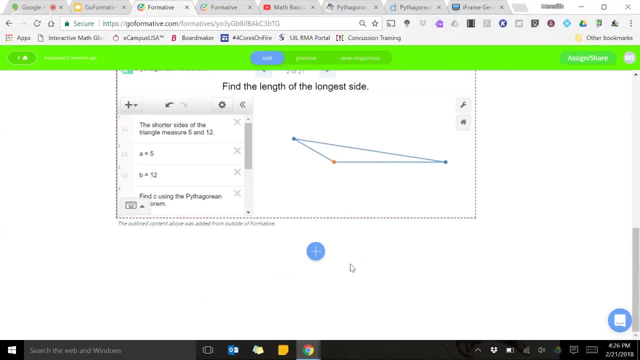 flipgrid, which is the video, and they can record themselves. yes, speakpipe and and um and vocaroo. basically, what you can do with those websites is you can create audio recordings and then you can embed them into formative. so, for example, if you, if a certain student benefits from having you know a question read to them, or you know a reading. 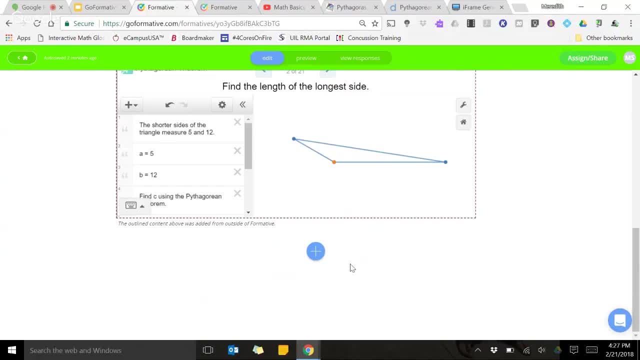 passage or like a word problem read to them or anything else. you can create the recording and then embed it into the formative so that they can listen to it as many times as they want. you know, and get that extra, extra support and that extra aspect of multi-sensory learning. yeah, that would. 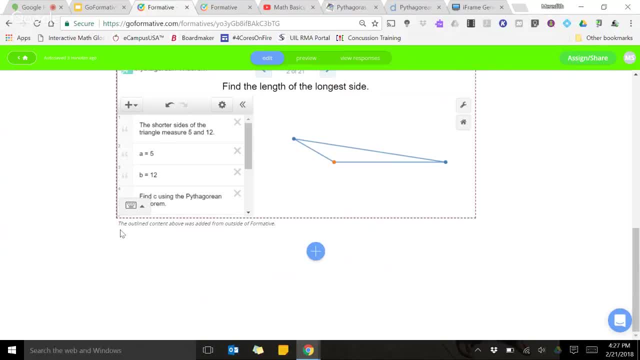 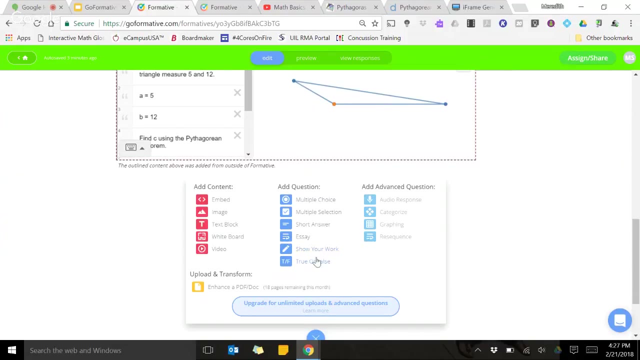 be really good uh for math, for my uh ell students or even for english language arts. that would be really good uh program to use. and then i think another one was the show your work is the one that i really wanted to do to show your work. so when you click the plus, 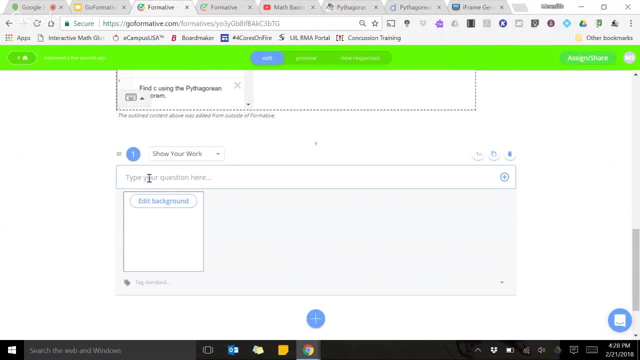 you just do your show, your work. so if you want to have them type a question or a direction, it can be right here. um, in addition, which i haven't mentioned yet, you can actually tag your standard. so i have mine set to texas. so if i wanted to tag my standard, i can do 8.7. 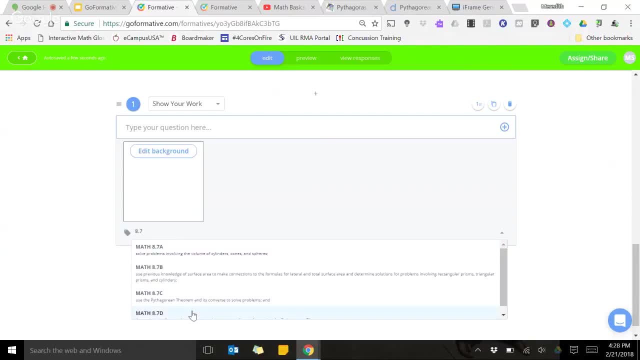 c on the pythagorean theorem. so it's tagged. so when i look at my tracker, i can see exactly um what standard i'm using. so i can see what standard i'm using. so i can see what standard i'm using. so i can see what standards they're doing well on or need help on. so to do the show your work, you just 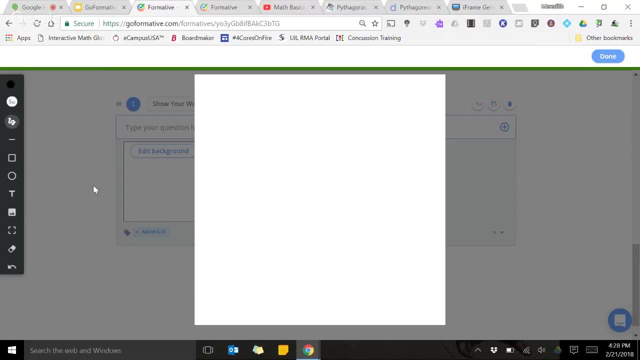 hit edit your background. if you wanted to, you could type something so you can type. and this is on the teacher side right now. so once you do this, the student can't change it. so if you type directions, they can't erase it or anything. if i wanted to upload an image like the one i showed, 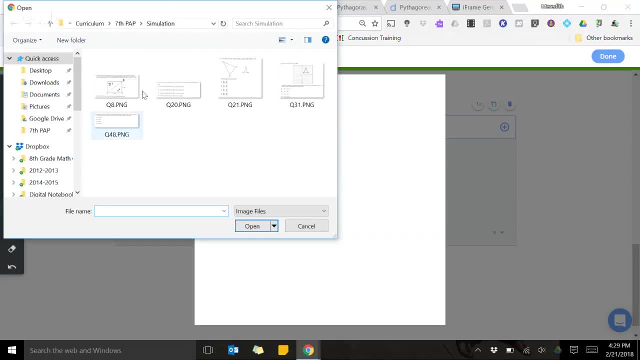 you today about doing the proportions is the first thing, and then i can just add a new one to this and i just want to make it easier for the students. so i can just say, like, we want this one to be bigger, we want it to be smaller, we want it to be bigger. you can take this up and then go ahead and drag it up and 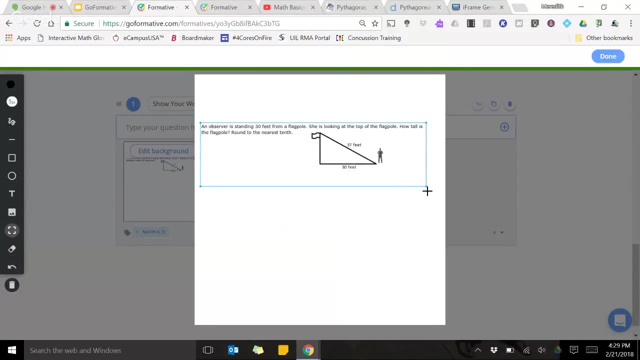 you can actually just take a look at your slides and drag it around and it's going to sort of do different things on the slide, so i can just drag it around and i'll just add it and it will look pretty cool. if you want any more, did you see anything else in the class? yes, no, if you want to. 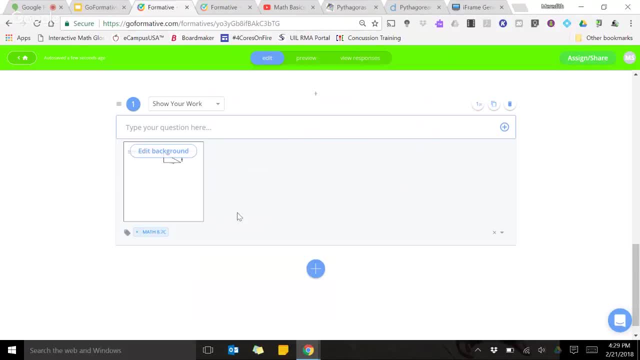 add that to your topic. please go ahead and start your class top of it and show their work on it. so that's one thing i really like about the show your work for that one, yeah, and so when you can also preview it. so when you're done you can preview it, and 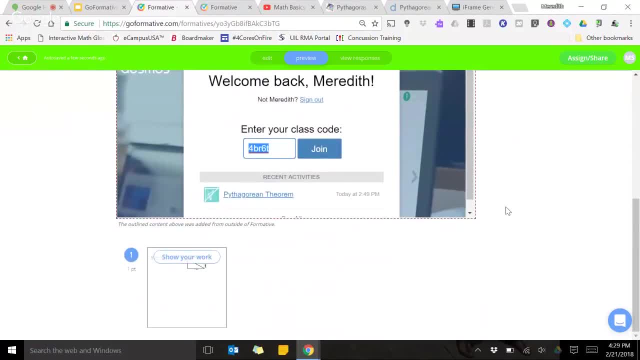 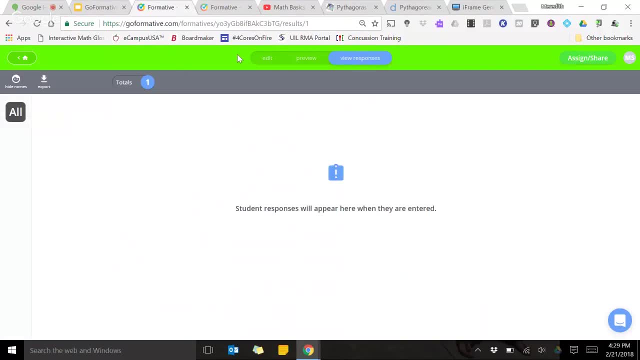 see what it's going to look like on the student side and then you can go over here and do the view your responses so once they start answering- or you've sent it, shared it- they can start answering. so right now i only have one question on the show your work, but you can hit the assign. 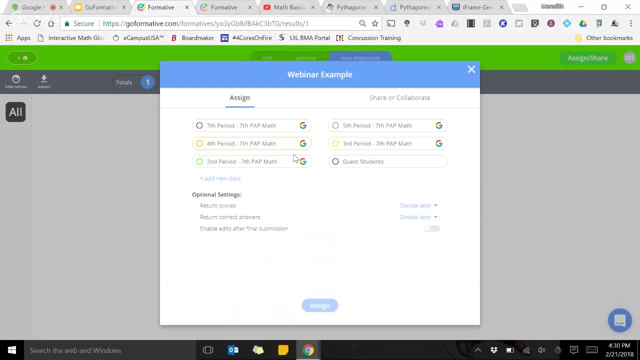 share button and it works really well with google classroom. so all of these classes were imported from google classroom, so i didn't have to add each student individually. it's all was imported, so i can just choose whatever classes i want. um, if i, i usually allow them to edit after submission. 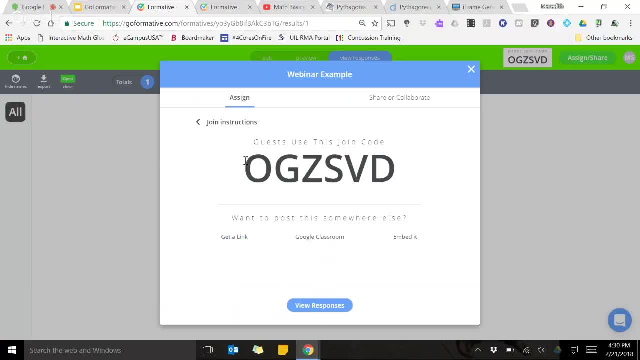 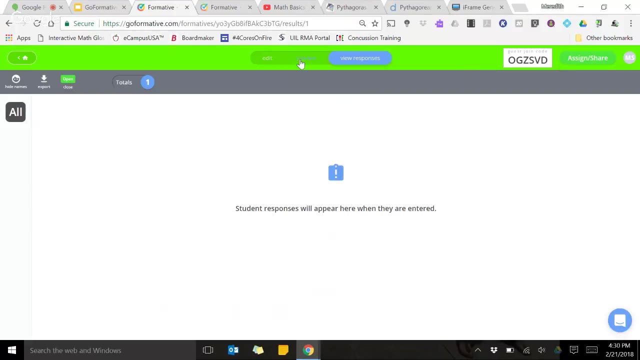 so they usually edit it and then you just assign and it gives you the option to have them do a join code or you can give them a link. so that's really easy how i i usually do the link on google classroom and then i just click on the link and it takes them directly to formative. so this is 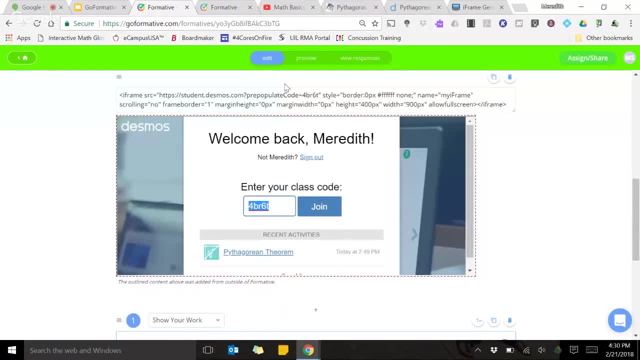 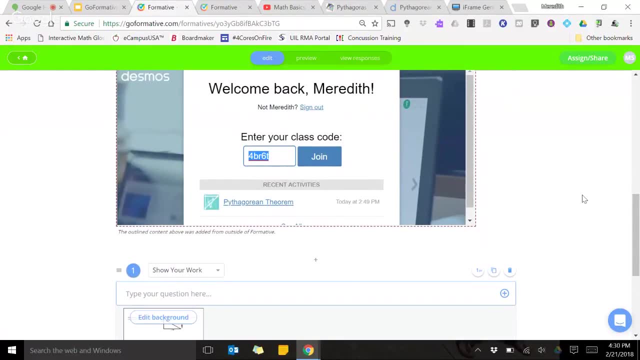 really easy way to get some lessons done, could i mention? could i just add one thing? um, i know tagging questions to standards and just to show everybody what that looks like, just in a, in a picture right here, basically like what we're looking at here is the tracker. 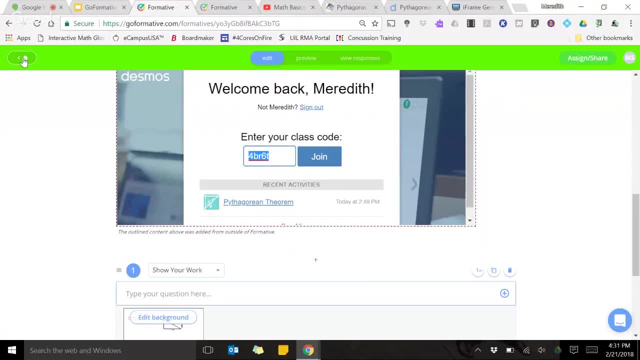 just an example of a tracker, and we saw meredith, you know, tag that one math standard. let's say that's this one, right here, you'll be able to see. you know, because you're tagging questions to standards. you'll be able to see how each of your students is doing on those. 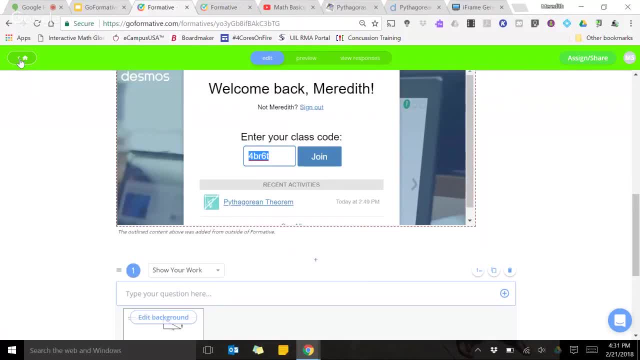 on each standard and so you can see, for example, cho here has a 75 average, you know, on her ratio standard and probably more, you know, if you're, if you want to drill in even deeper, you can click in and, uh, you know, actually see a student's response for every standard. so 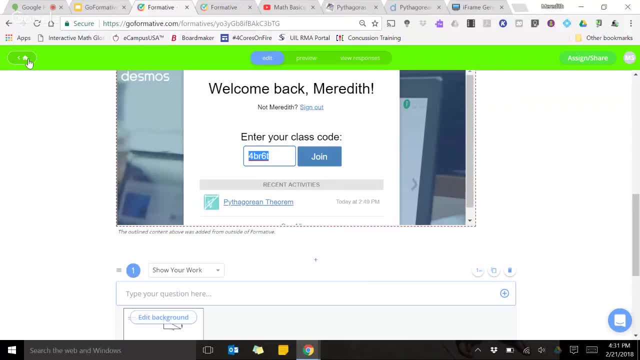 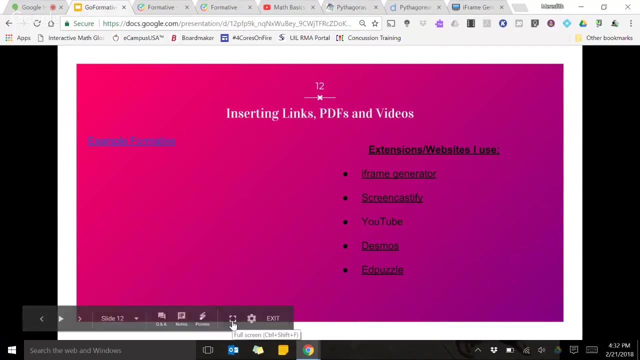 we're looking at dean thomas and we're looking at his, all of his responses for for any given standard. so you can, you know, not only see what he needs to work on, but also, like, look at that whole portfolio and figure out how you can support him. so that's, that's. that's it. 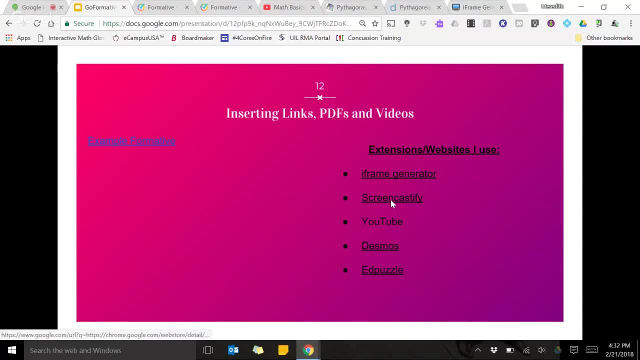 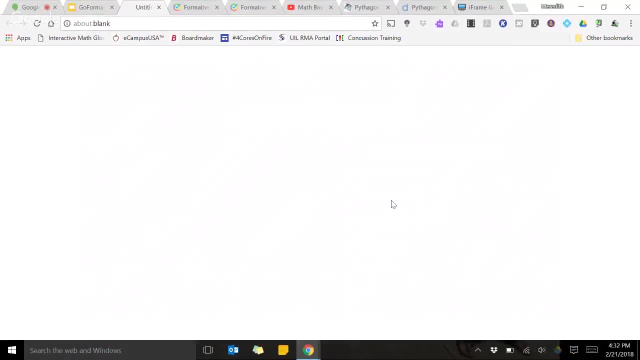 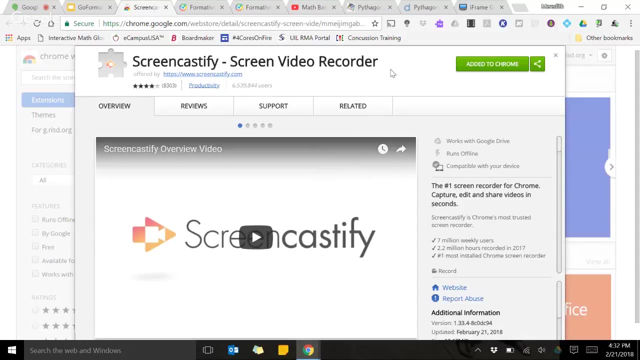 and then so, and the last thing i just kind of want to go over is: it's a. this is how i make my own videos. it's the screencastify. so if you click on it, just go to the google web store. it's called screencastify- screen recorder. it's free for up to if you want to. 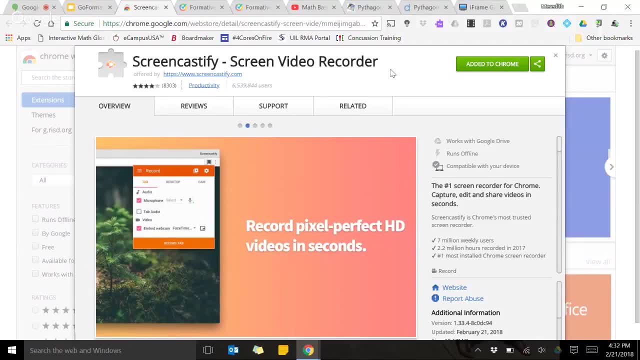 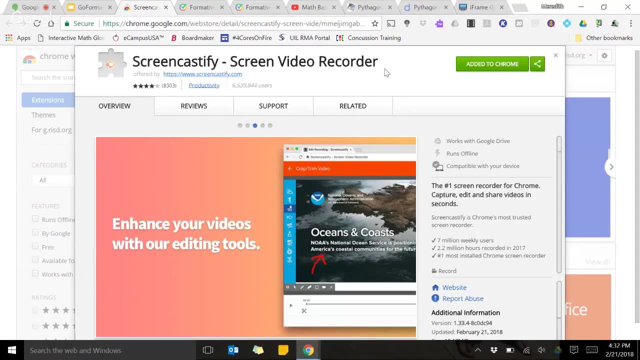 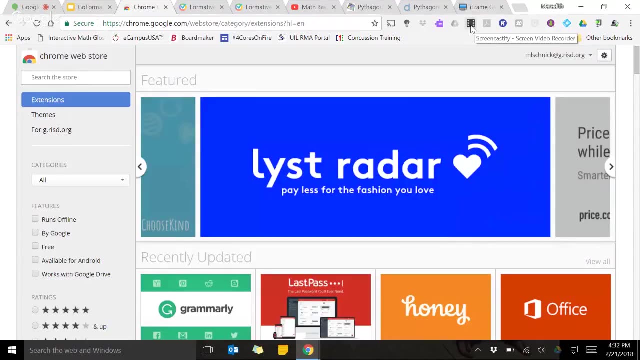 record videos up to 15 minutes. i usually only do like short four minute videos because the kids can't really watch anything for longer than five minutes. um, so mine's already added. once you add it, it's this little uh film strip right here. that's up here, and once you press it. 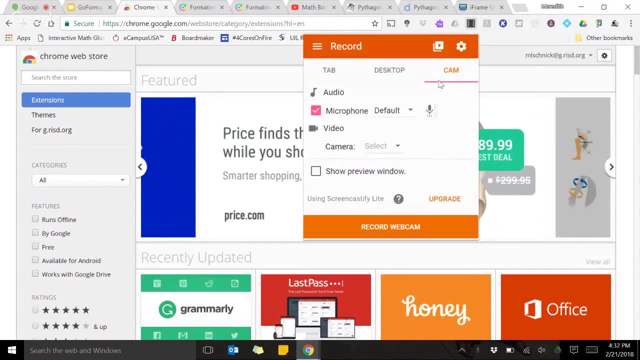 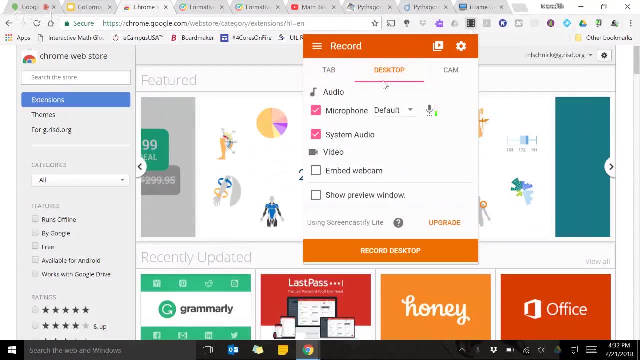 it actually gives you the app option to either do a video camera- you can just record just the tab that you're on, or you can record your whole entire desktop and it records it and then it automatically saves it to its own file in google drive. so if i go to hit the little three bars, 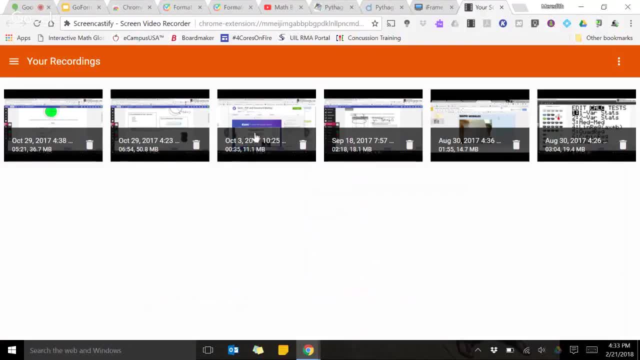 and go to my recordings. they're all here that i can upload. so that's another feature. and all of these, every time i create a video, works perfectly with formative. i can import it into my formatives just like a youtube video, just like this video up. 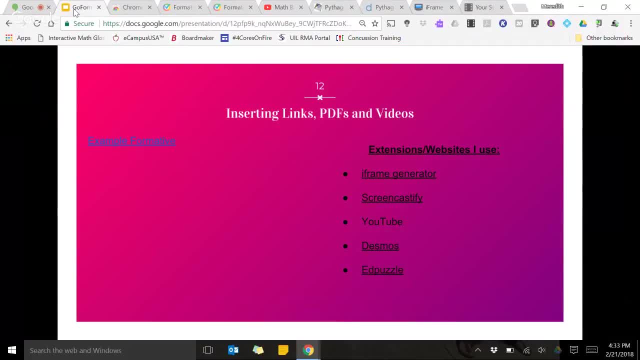 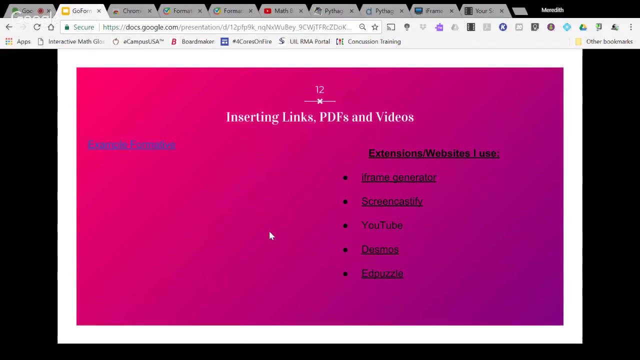 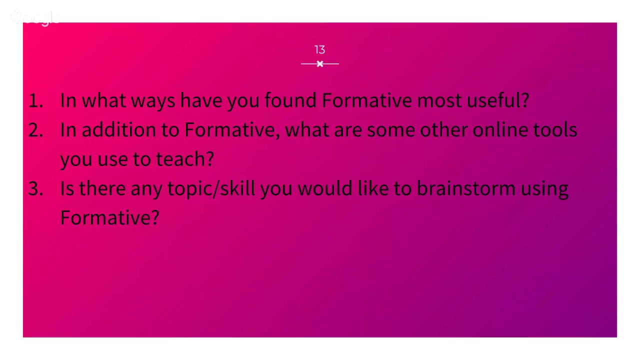 here, where it's right there on the same screen as well. so that's what i love about everything: everything's so compatible with formative that i can use other programs and extensions on there. awesome, cool, yeah, and then just any other some questions if anyone's used formative. 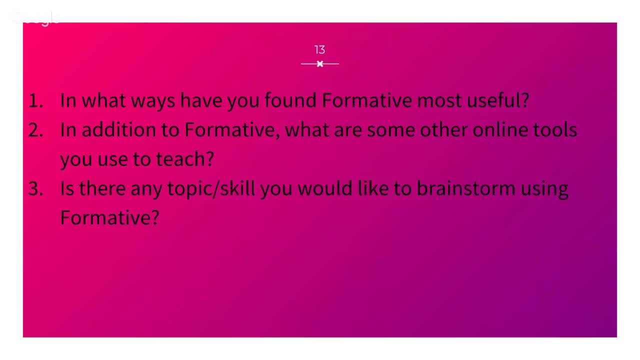 uh. what ways have you found for formative most useful or what are some other online tools you used to teach with using formative? i know we mentioned the uh geogebra and that speak pipe. i didn't know if anybody had any other online tools that they use within formative. 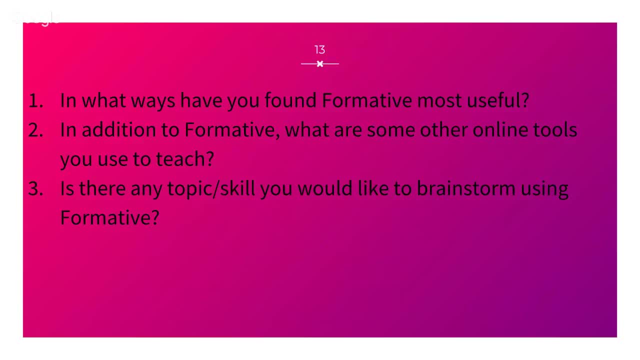 um- and i know- that's one of the many things that i've learned from here- that our program is pretty innovative with some of our other courses. so i've done some pretty good work with the uh conversations with our other students and we looked at a lot of different things we've done. 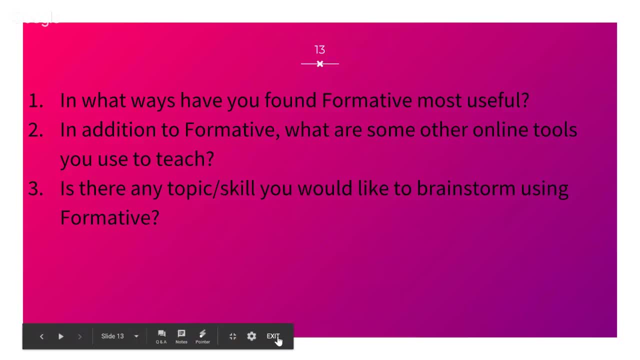 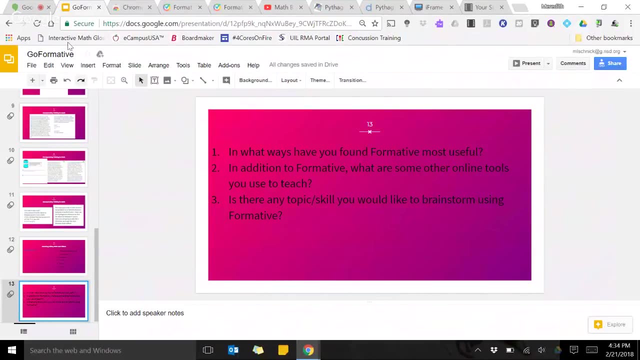 about how to make sure that students can have some fantastic experiences with the program, and So, yeah, I'm sorry, Did you want to share your screen so you can show them the community center? Yeah, I think I'm on it now, Okay, Uh, no, Oh, there we go. Now I can see Gotcha, Uh. 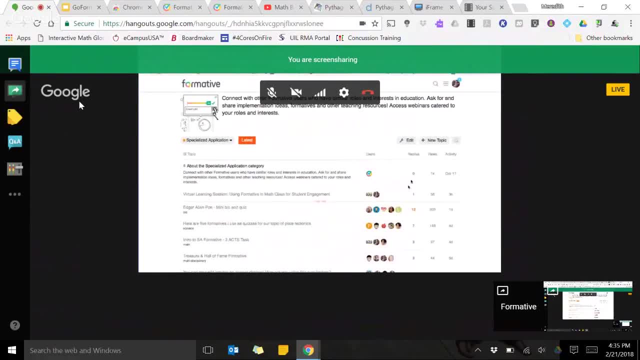 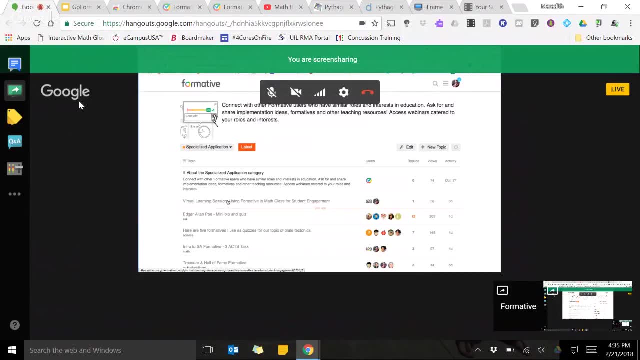 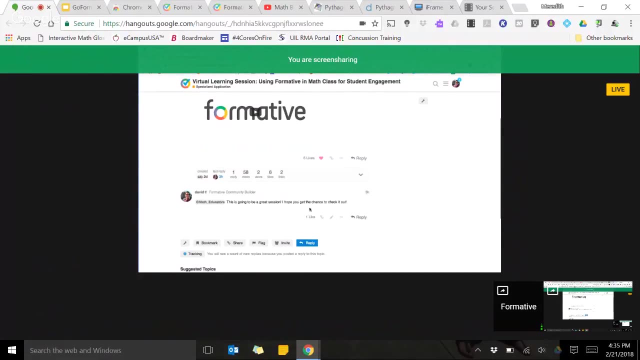 cool, Um so so, uh, this is the community center right here, and you're going to see that, um, Meredith's uh topic is right at the top here, And so we can probably just include the questions in here. right, Meredith? And that one, you know you're visiting our community center. 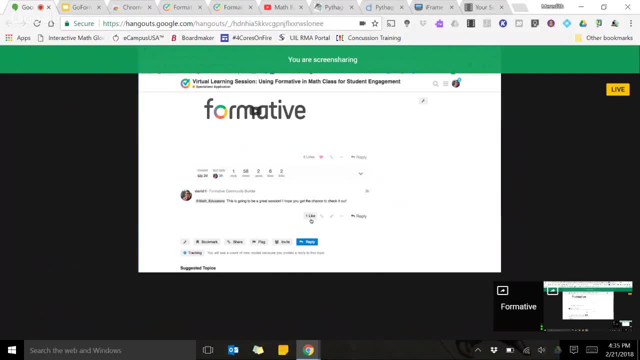 You can join the conversation and and share your responses to her questions, or just share any feedback you have about, you know, her webinar, So so, yeah, But uh, yeah, it's just discussgoformativecom to get to the community center. You can also. 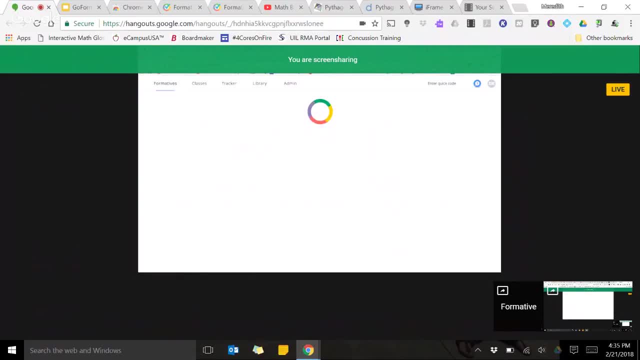 access it right from your formative dashboard. So like, if you just signed up for the community center, you can access it right from your formative dashboard For an account. it's always going to be right here, uh, community center, and it'll actually. 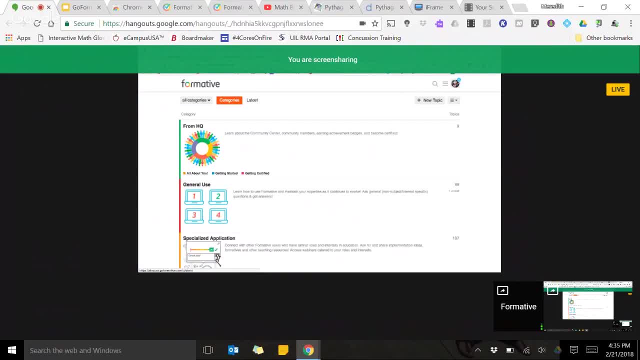 just log you in based on your formative account And you'll be able to collaborate with so many teachers. uh, in here. You know I met Meredith through here, which is so cool that we were able to do this together And it's it's all because you know we connected. 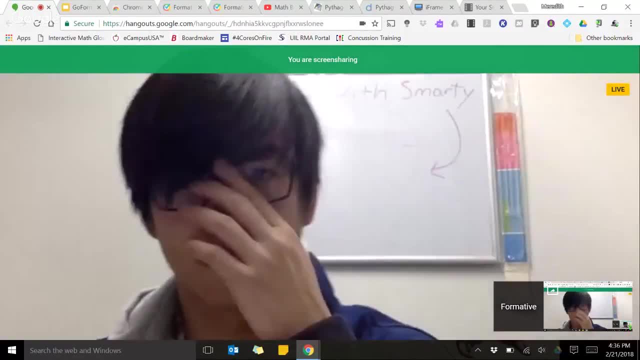 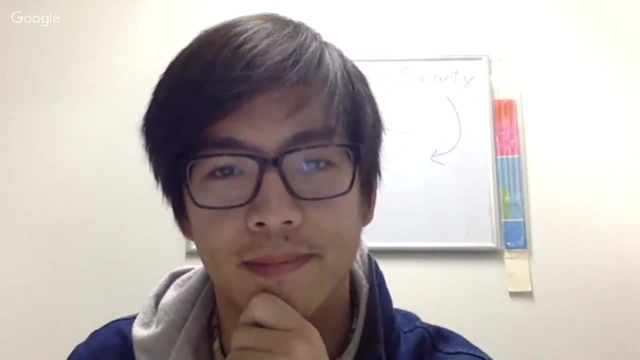 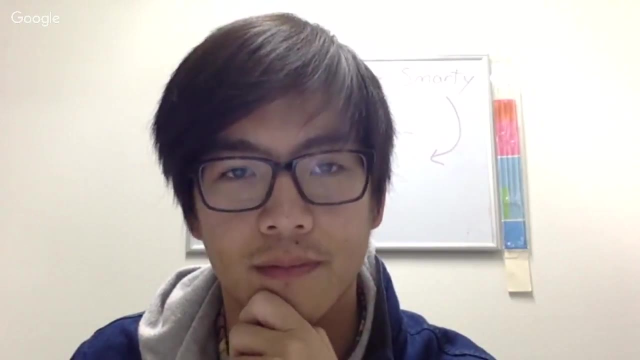 And a lot of the programs that I found uh. for example, the iFrame generator was through the community center where I watched another video on the uh tips and tricks. I think it was uh, the tips and tricks part one, And so I was just watching that webinar on the formative. 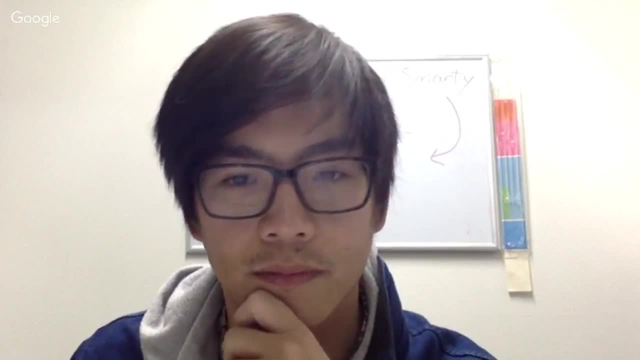 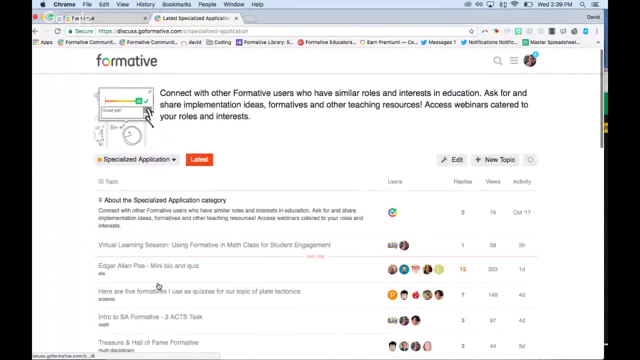 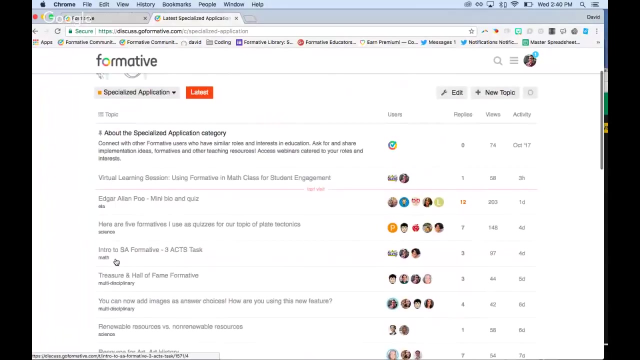 and figured that one out. So there's a lot of uh good examples, even lessons, on there that are free to look at. So that's one thing I really like about it. Yeah, Just to show everybody that, if you're interested, there's all these tags right, For you know different subjects, So 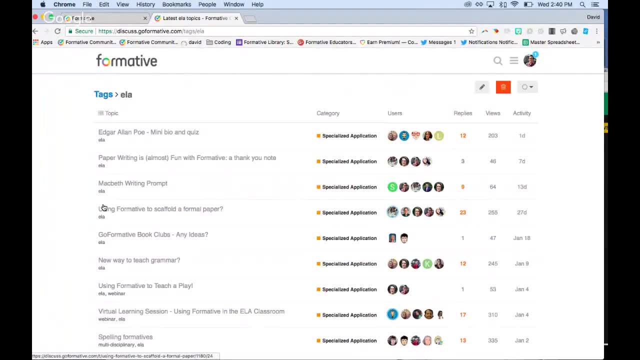 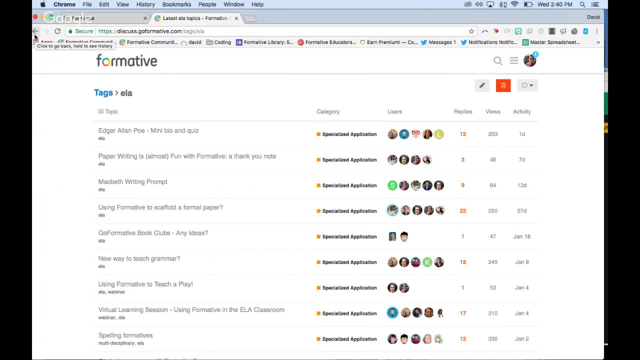 if you're looking for subject specific resources like ELA, you're going to find a lot of great conversations in here just around ELA and using formative and other tech tools for ELA. And then same thing if you're- if you're looking for all our webinars- um, there's a tag for webinars here. 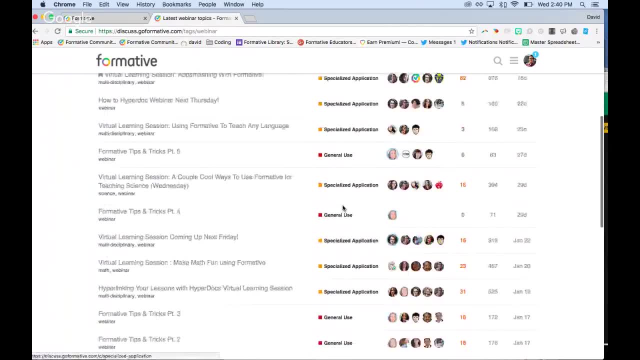 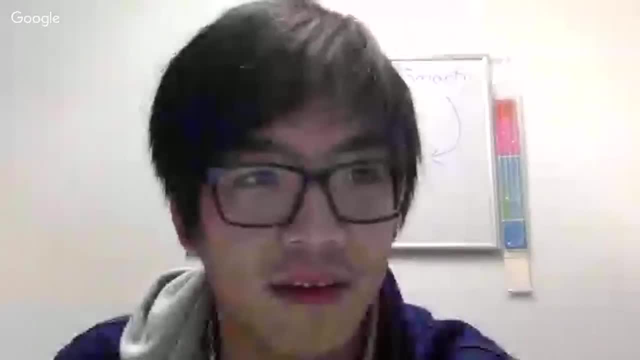 too. So if you click on it, you're going to, you're going to find all of our webinars. Um, like I said, they really range across the board. So if you're looking for, if you're looking for different uh subjects and just uh, different interests that you might have, 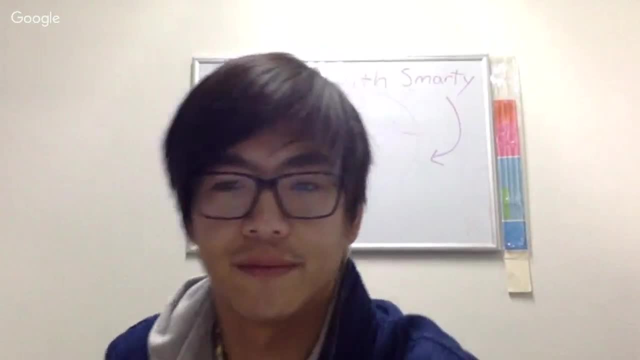 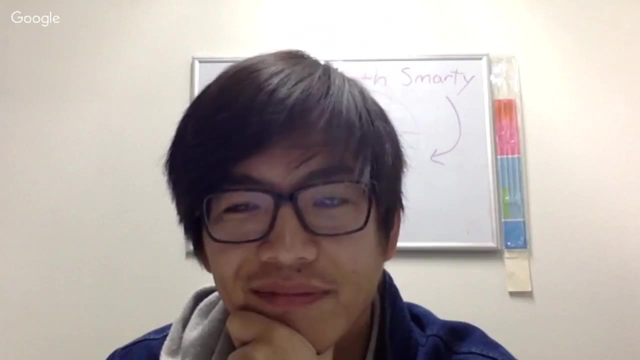 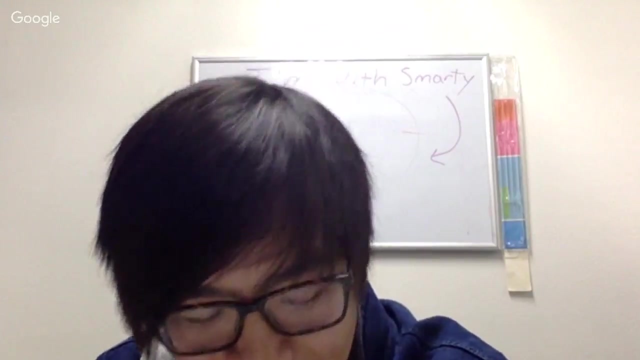 And I started with the tips and tricks, one and that one. that's to start with part one, part two just to get, uh, introduced to a lot of the other features. So that was really helpful, Awesome. Well, Meredith, I want to definitely thank you for rocking an awesome presentation. 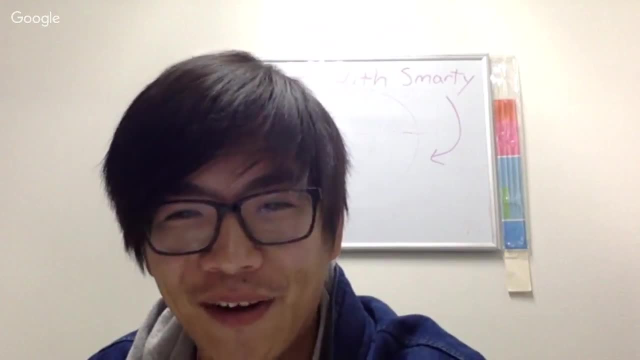 Really, really, really enjoyed it, And I think we both like to thank everybody who tuned in out there and for sharing your questions too, And I hope you got a lot of great ideas out of this. Did you want to say anything, Meredith?